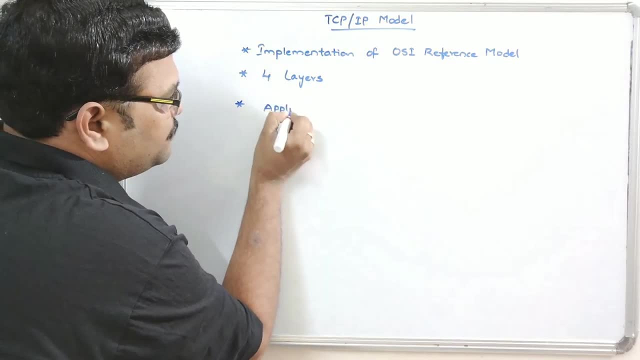 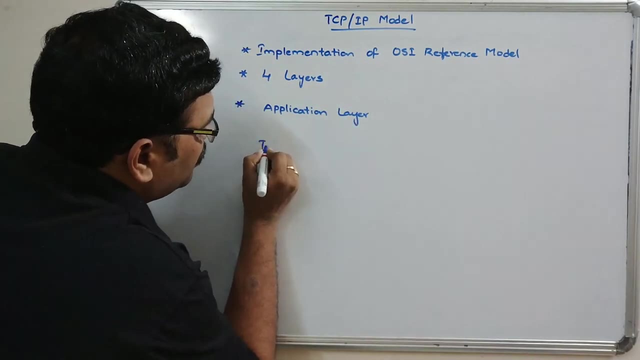 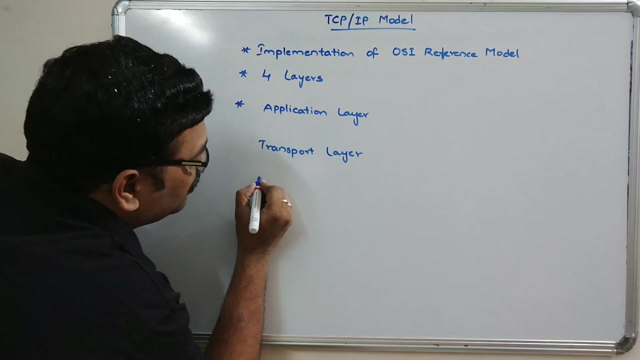 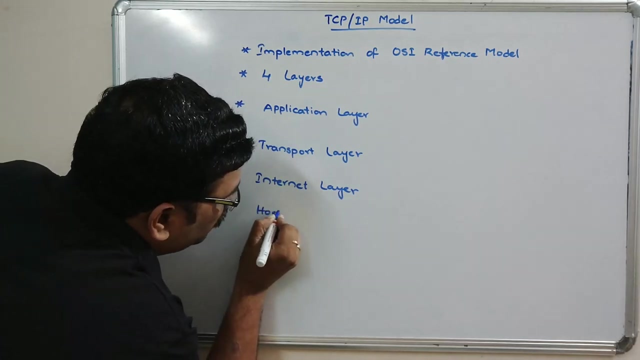 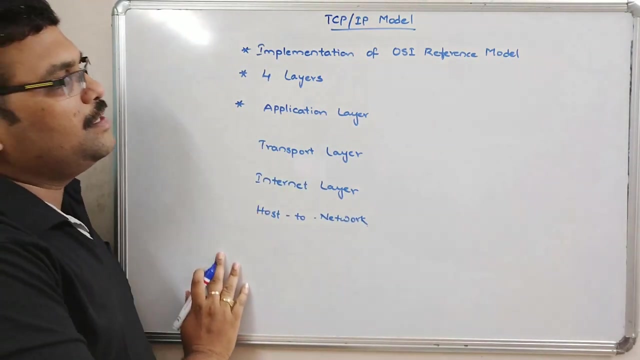 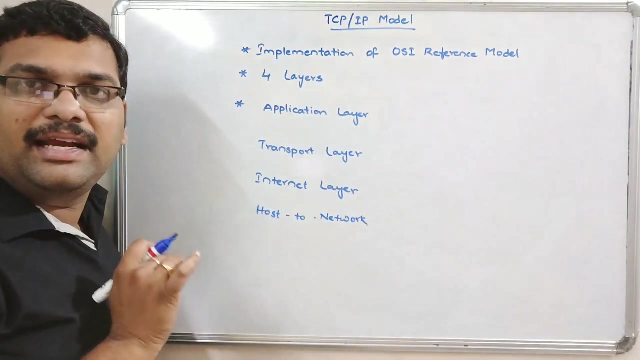 four layers are: the application layer, translation layer, application layer, application layer, transport layer, internet layer, host to network layer. So these are the four layers in TCPIP model. So let us see what is happening in each and every layer: The same thing, but 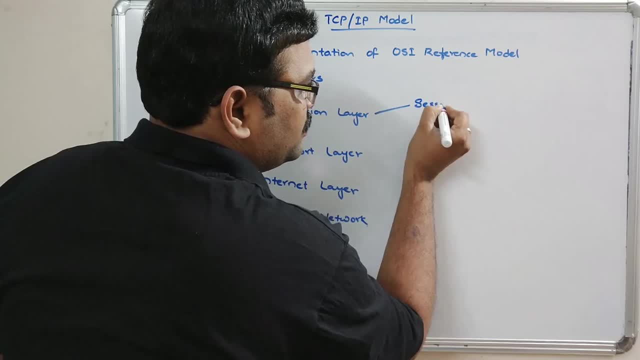 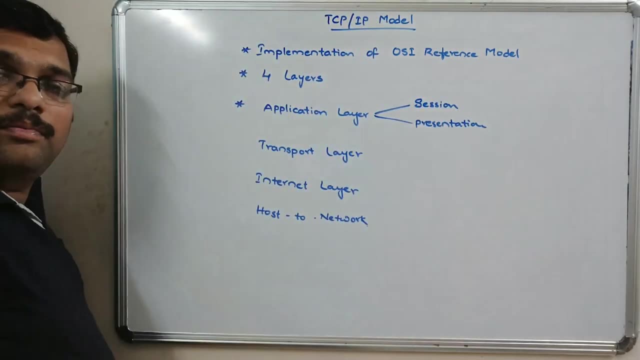 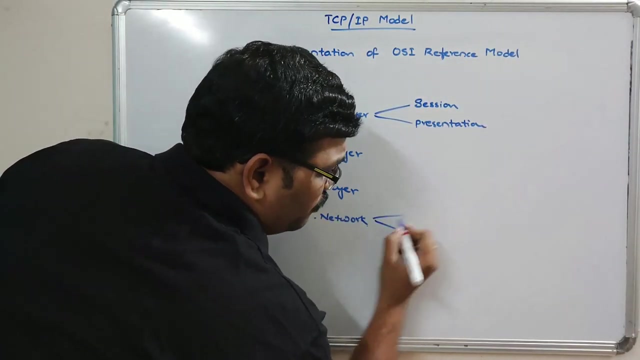 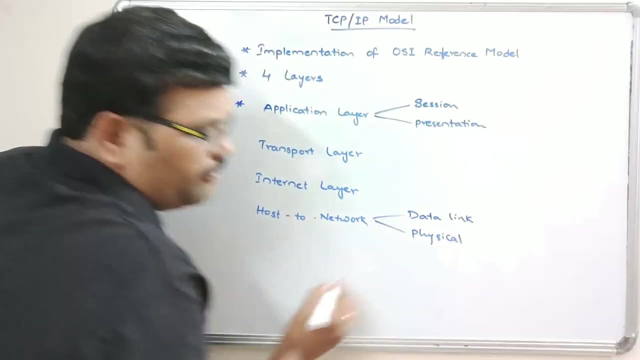 in the application layer, we are combining the session and presentation, So combining these two layers in the OSI model. in this application layer, And coming to this host one, we are combining a data link layer and the physical layer. We will combine both the data link layer and physical layer of OSI model into a single layer of OSI model. So we will have a layer called host to network layer in TCPIP model And this is, as usual, transport layer and this is network layer. So this is the OSI layer and this is the TCPIP. 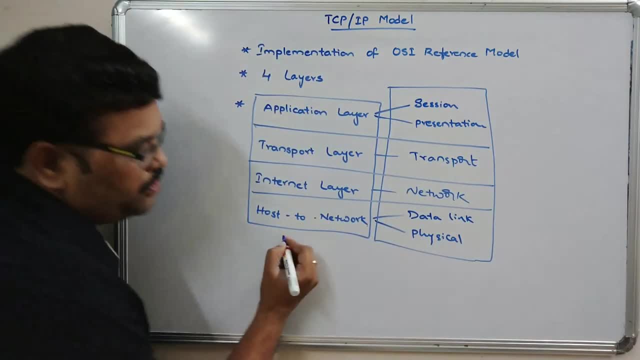 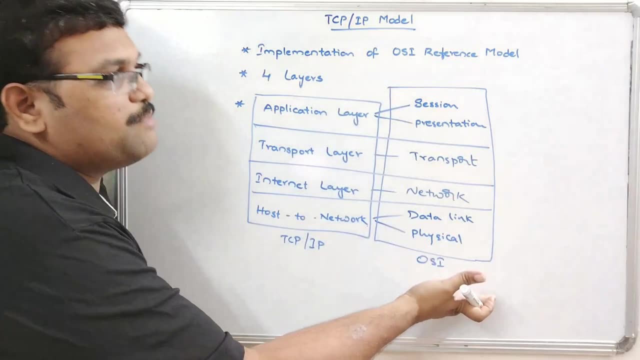 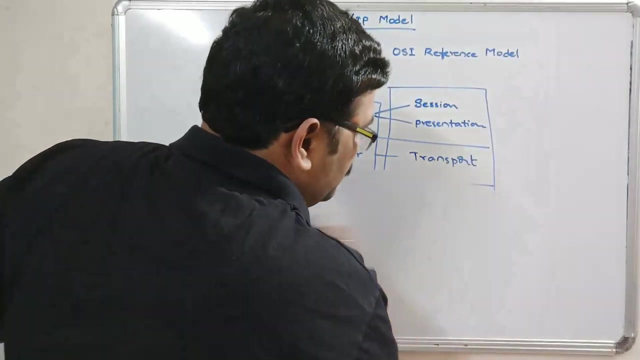 layer Right? So this is the TCPIP layer And this is the OSI reference model. So, implementation of this OSI model. we will get this TCPIP. Now we will see one layer after another, So let us start with the lower layer, that is. 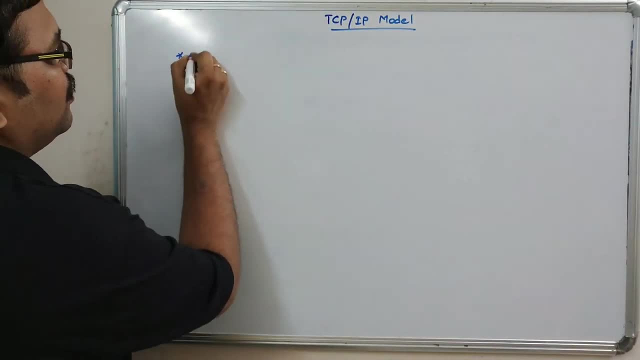 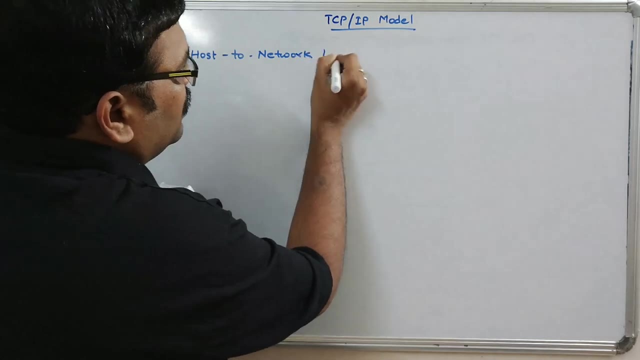 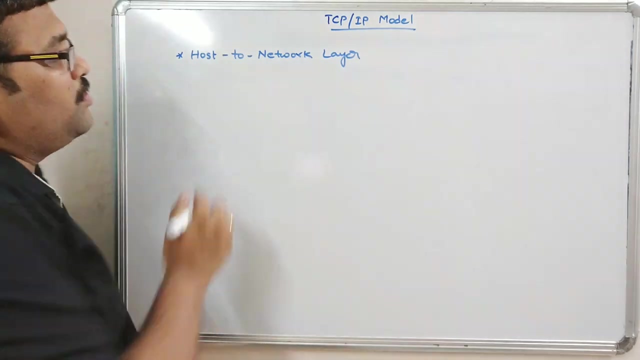 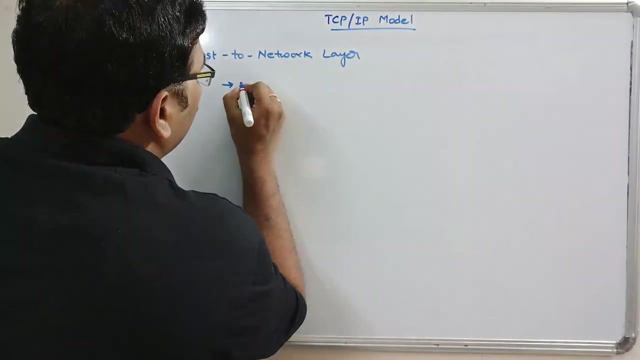 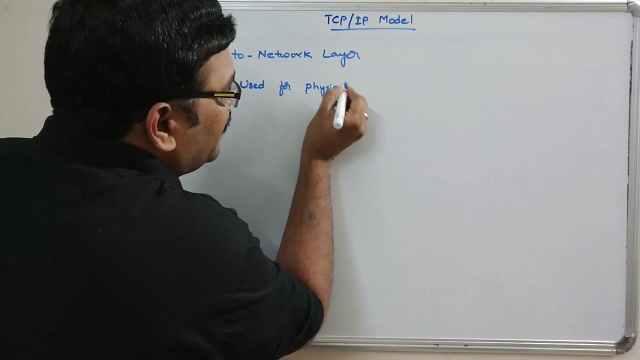 host to network layer. Host to network layer. So this is the OSI reference model And this is the jakby that we have written down. Let us take a look at this IIO as a language, And we will call it the First Boston. 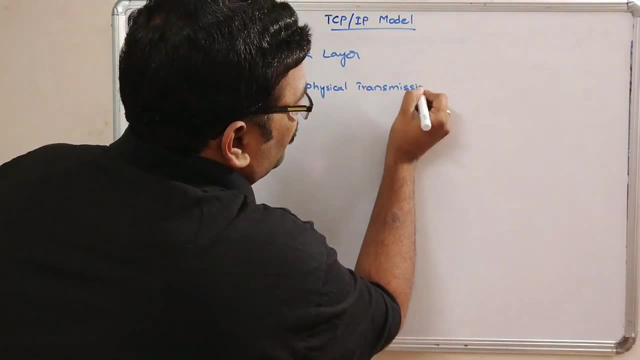 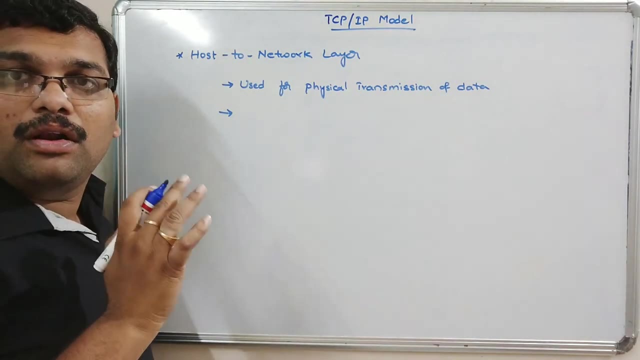 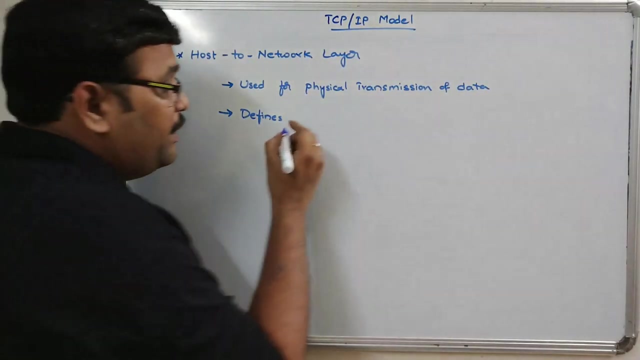 The first one I will use isly cái, The first layer here, First layer here. So this layer is unusual. This is slightly unusual. Right defines a protocol to connect the host. this layer is responsible to define a protocol. here. the protocol means a set of rules, so there will be some set of rules to be followed. 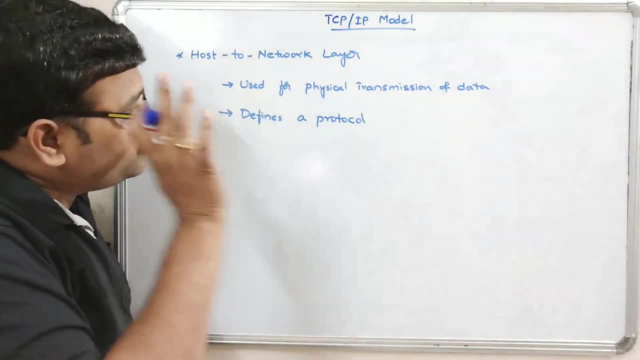 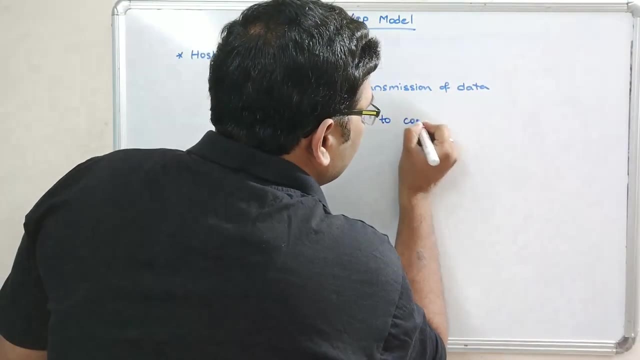 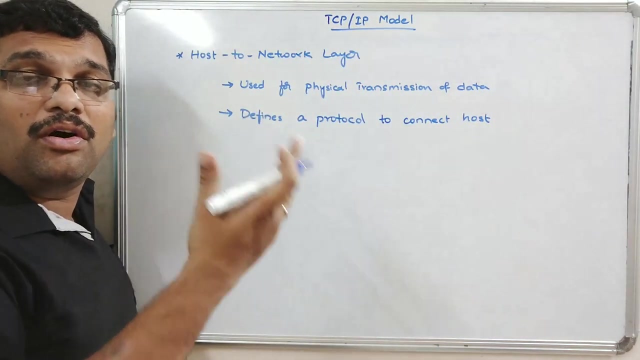 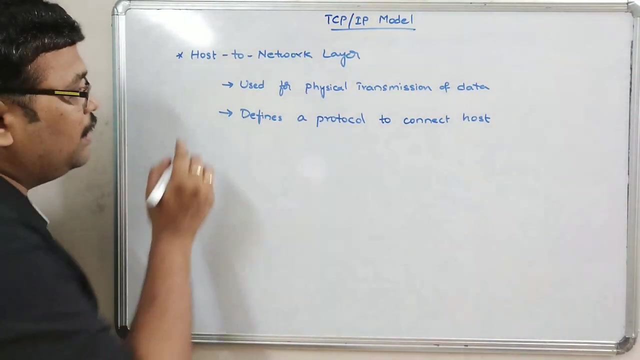 while transmitting the data from source to destination, so that protocol definition should be done to connect the host. so it defines a protocol to connect host and these protocols may be different from host to host or the network to network, right. so these are the things happen in this host to network layer and the next second layer, the layer the above. 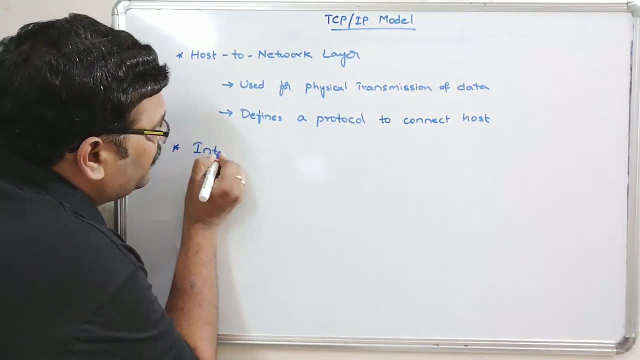 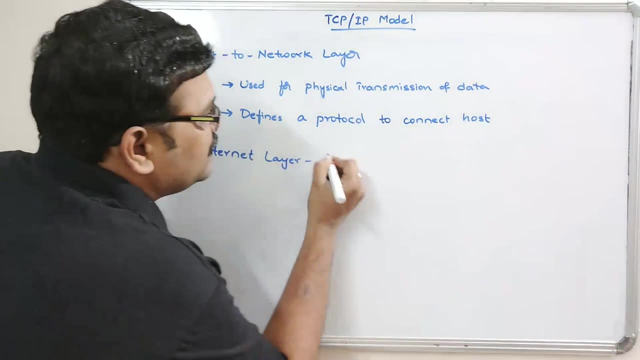 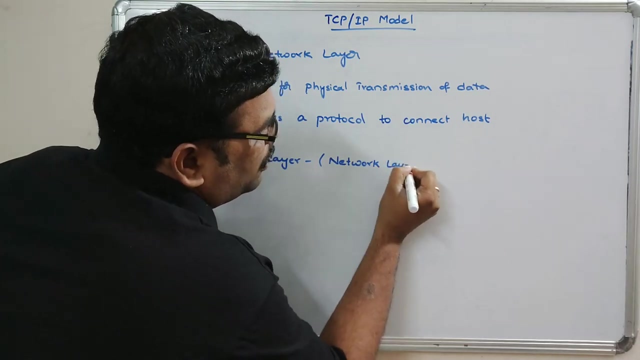 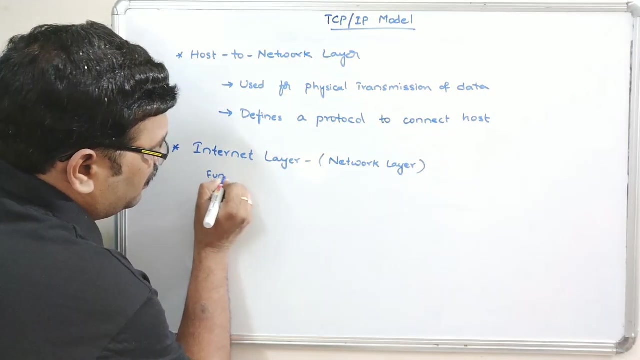 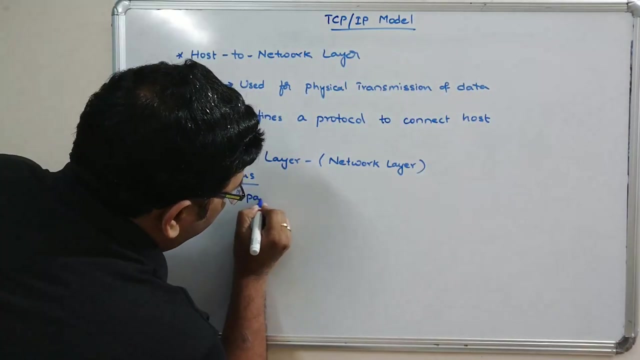 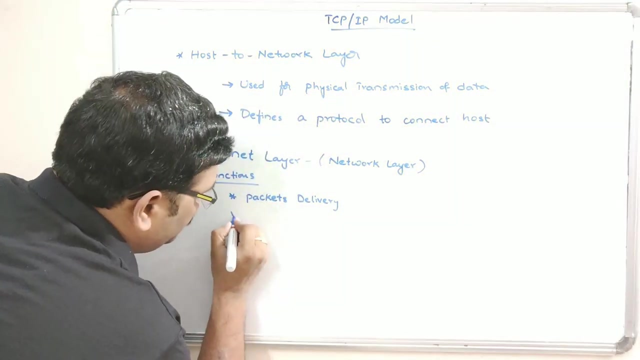 layer of this host to network layer is inter network layer or internet layer, right, so this is nothing but our network layer in OSI reference model, right? so here the functionalities are. the functions of this layer is packets delivery, so delivering the packets from source to destination. routing, so the packets will. 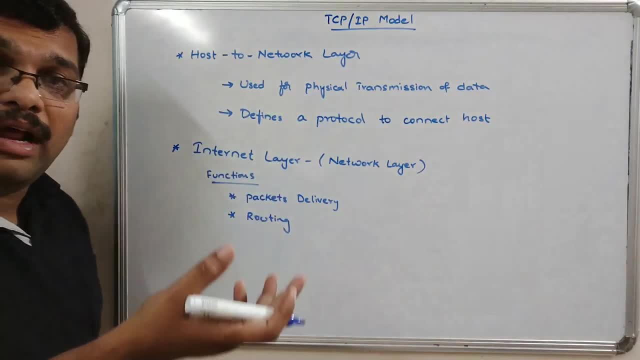 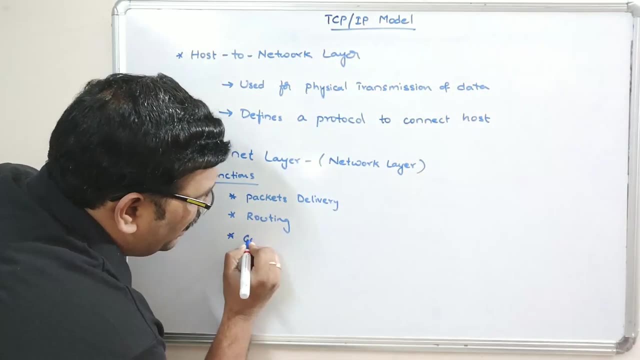 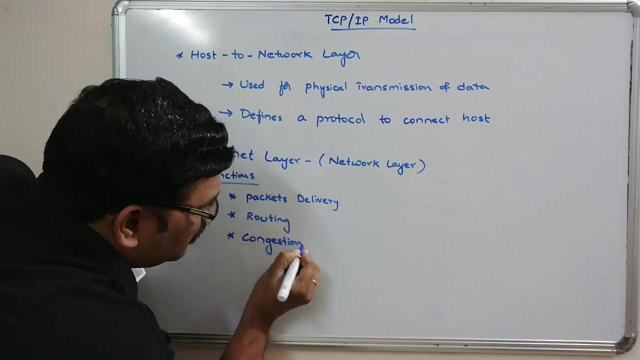 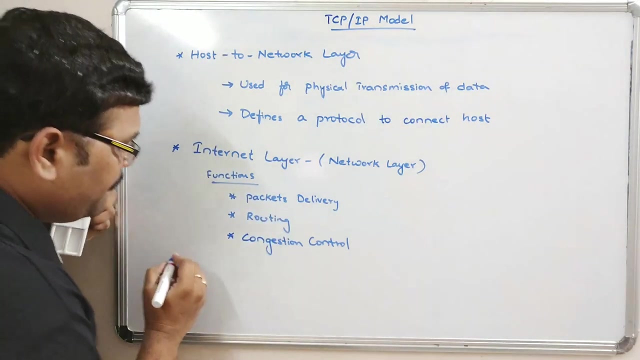 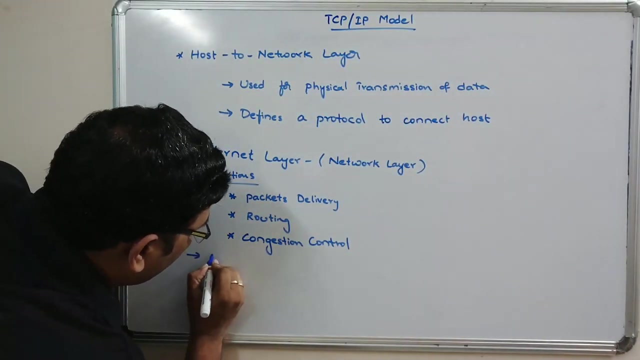 be routed from source to destination. so there, we will use some more algorithms for routing so that routing will be. routing is one function of this layer and, similarly, avoiding the congestion or congestion control, so congestion control. so in order to avoid these congestions, this layer is responsible and also the main protocol which is responsible for this layer is the. 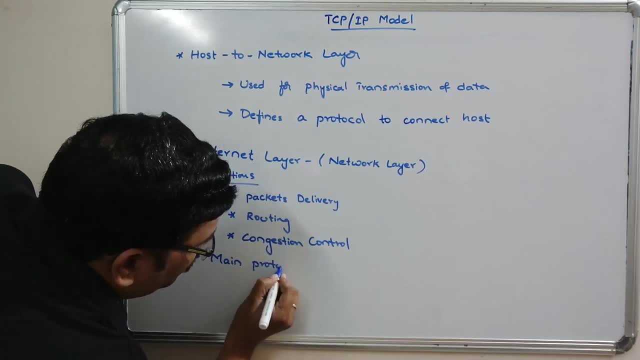 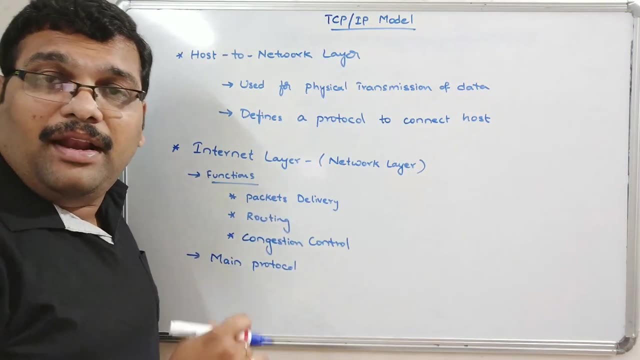 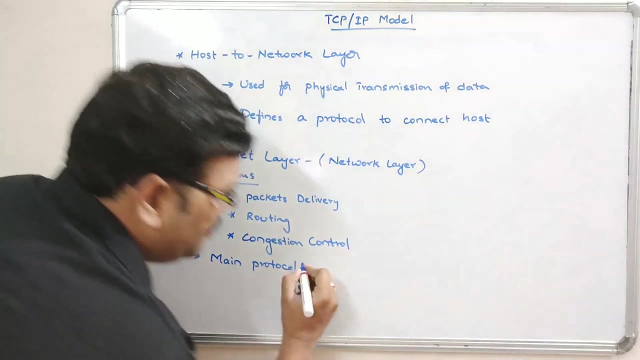 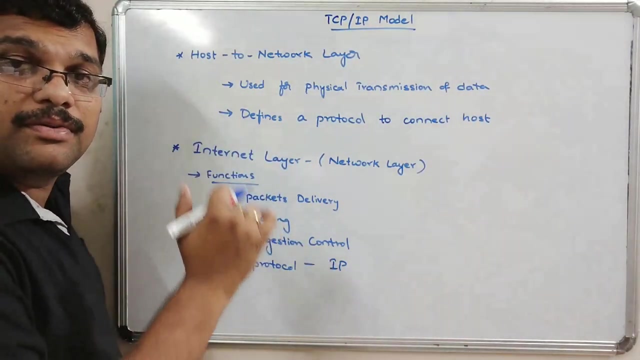 protocol of the host. So in the TCP, IP, the main thing is a protocol. so each and every layer will be having the protocols. so the main protocol of this layer- that means internet layer- is IP protocol. that means internet protocol, right. so this is used to transfer the packets from source to. 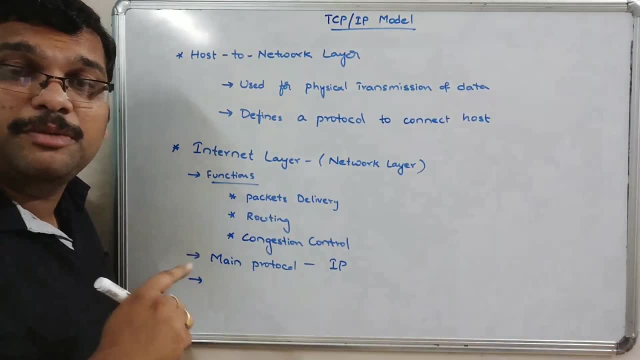 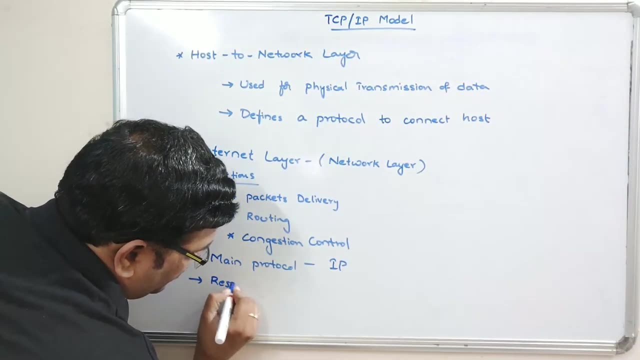 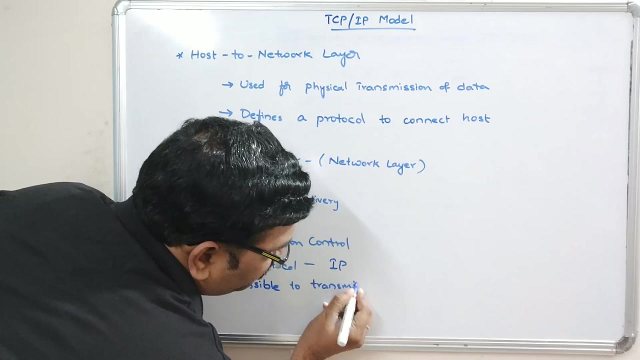 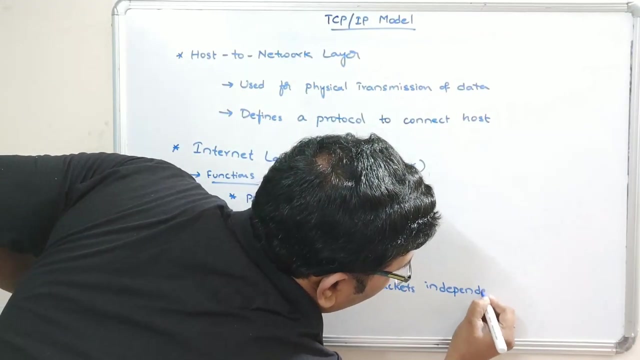 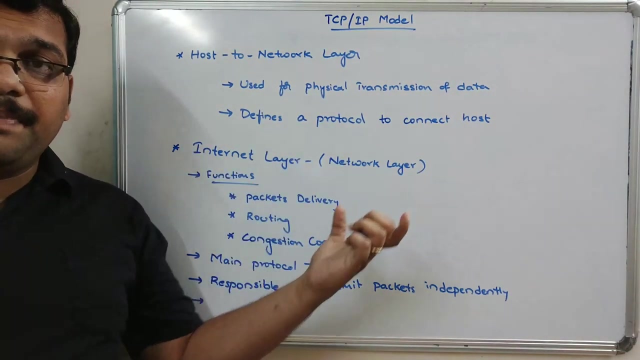 destination. so, and it is also responsible to transmit the packets. independent geosystems- right, so it is basically The responsible to transmit packets independently. So here this is responsible for transmitting the packets right so from source host to destination. so this layer is responsible for transmitting the packets right so from source host to destination. 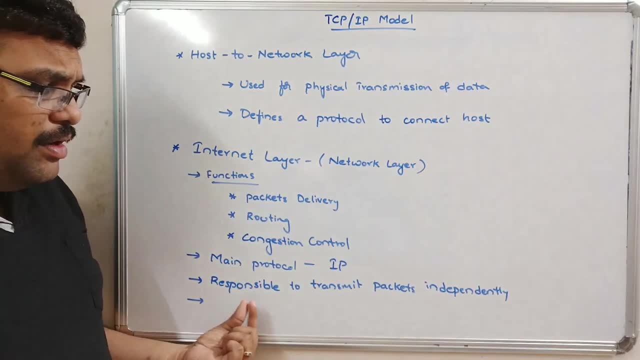 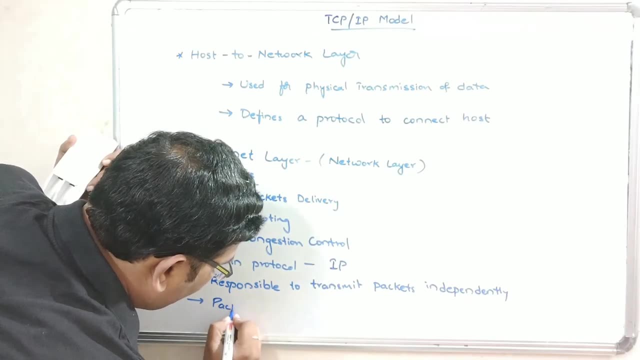 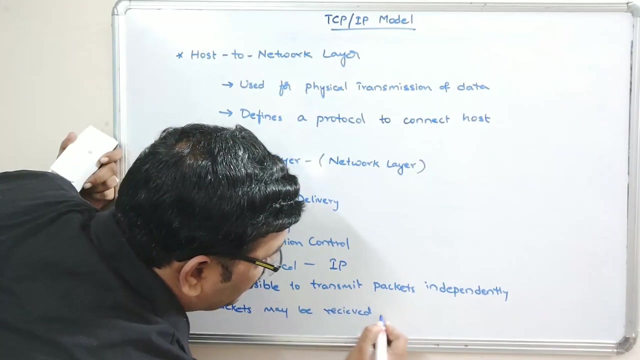 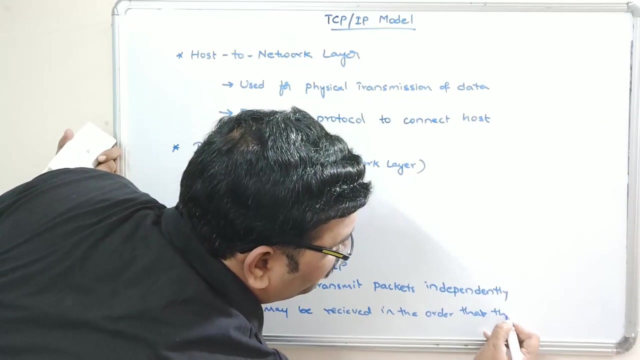 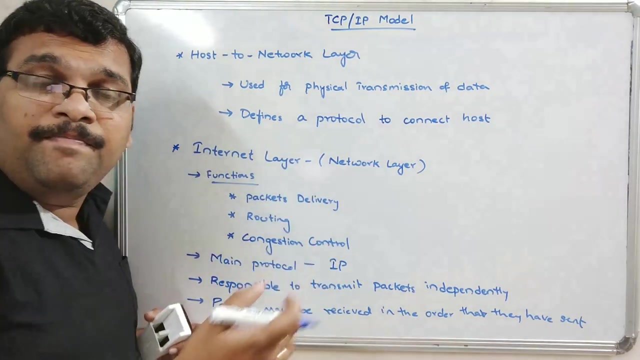 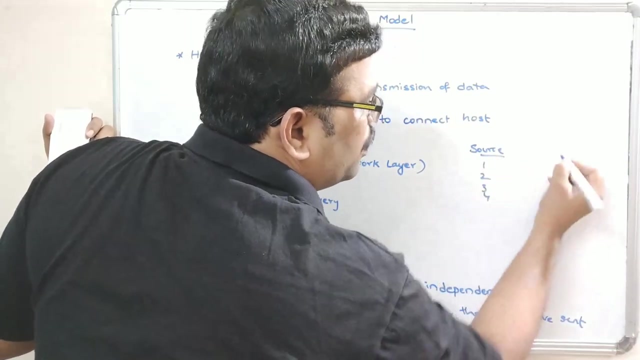 host. and again here, the packets may not be received in the same order that they have said. so the packets will be sent from the source to destination. so if the packets order from the source is 1, 2, 3 & 4 and in the destination, it is not mandatory to receive. 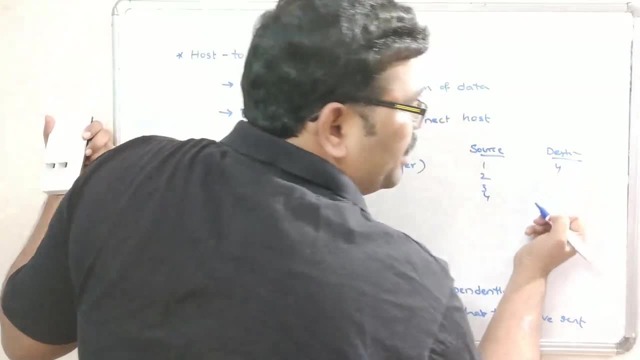 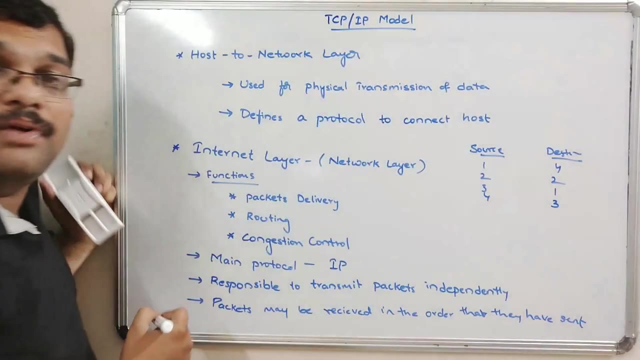 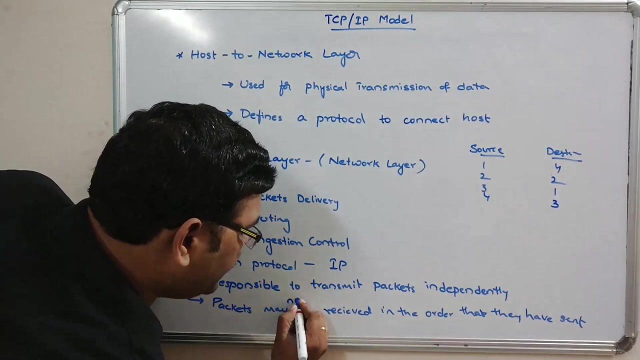 the packets just as 1, 2, 3, 4. so the fourth packet may receive first. second packet may receive second packet. number one may receive third packet. number three may receive fourth packet. number three may receive at the last. so packets may not be received in the order. 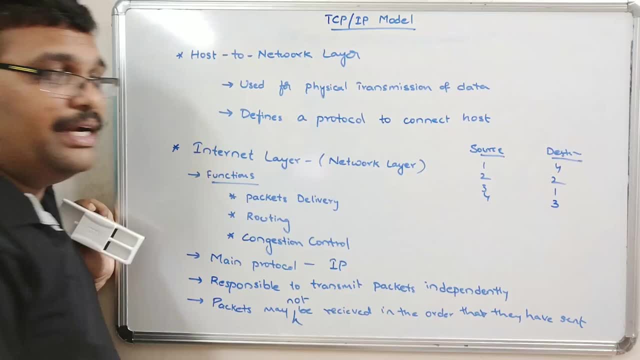 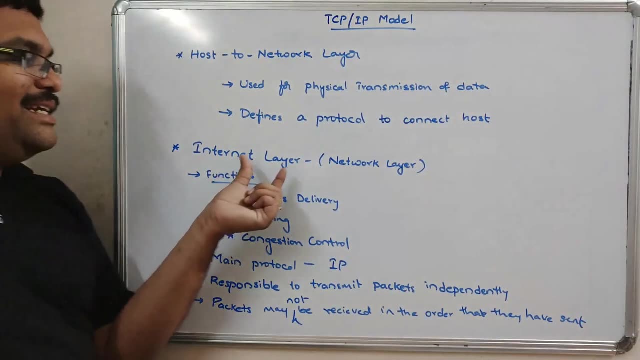 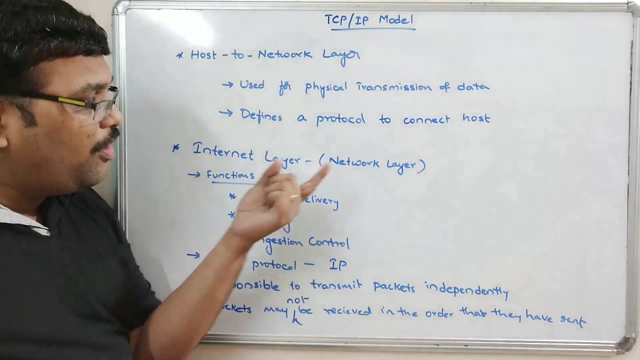 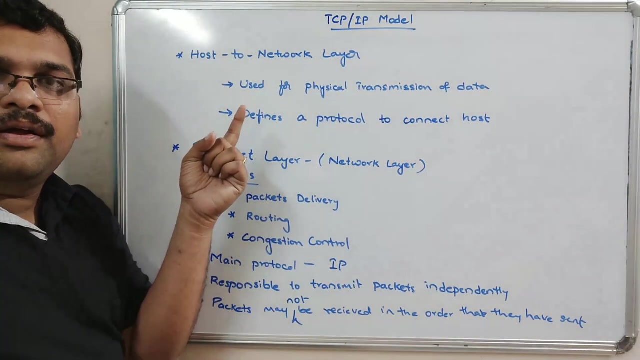 that they have sent. so whatever the order they are sending, the same order may not be received in the receiver side. so this is one more responsibility of this internet layer. so whatever the functionalities, whatever the responsibilities we have seen in OSA reference model of network network layer, everything is applicable for this internet layer in TCP IP model. right, hope you. 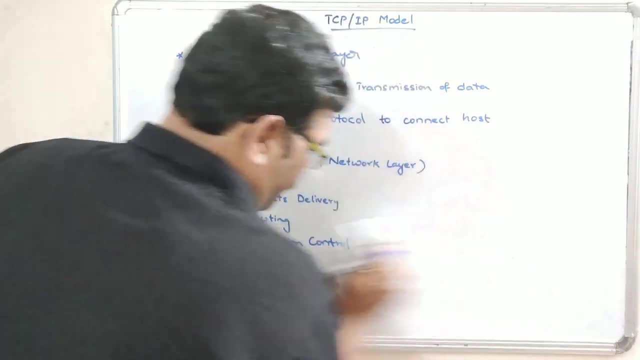 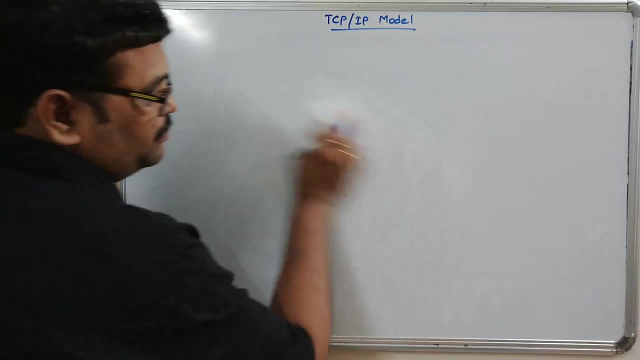 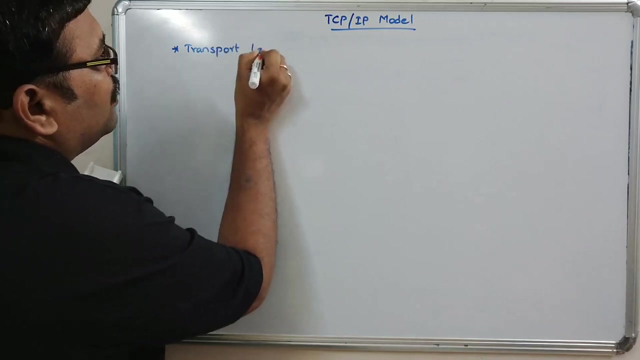 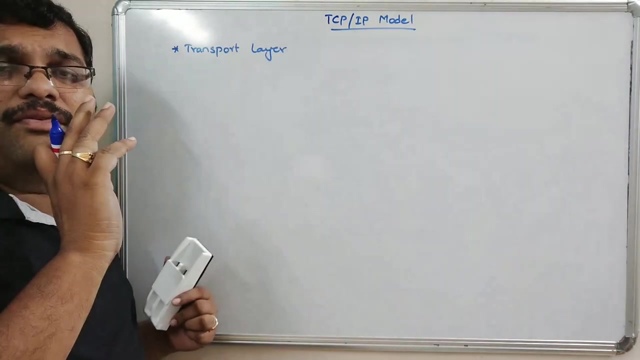 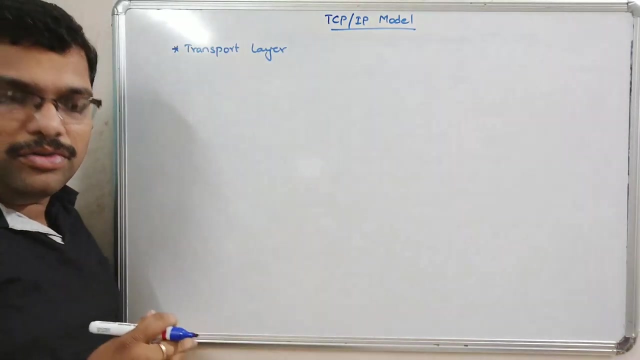 understood. next we will move on to the next protocol or next layer, that is, transport layer, transport layer, so here the transport layer. so same the functionalities. and whatever the functionalities and responsibilities we have seen in the transport layer of OSI model, the same will be applicable here also. the main function of this transport layer is: 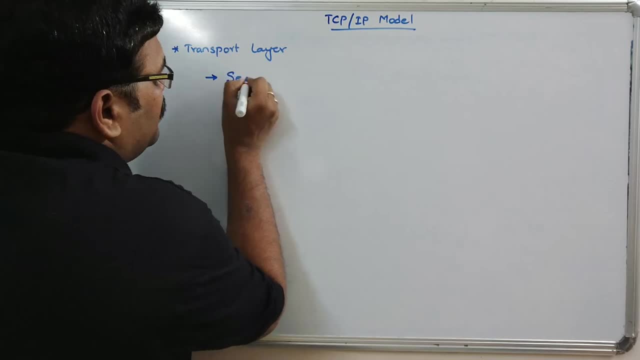 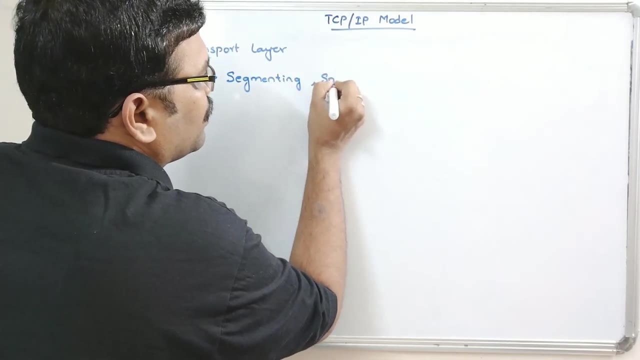 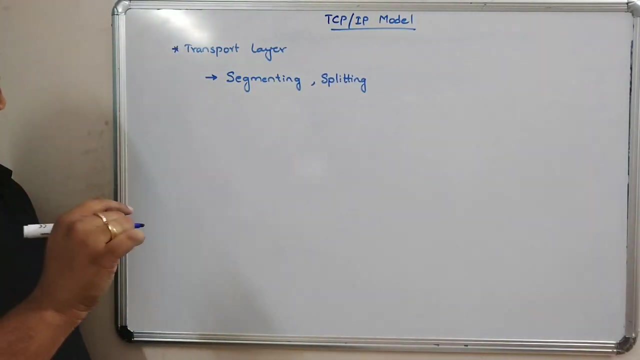 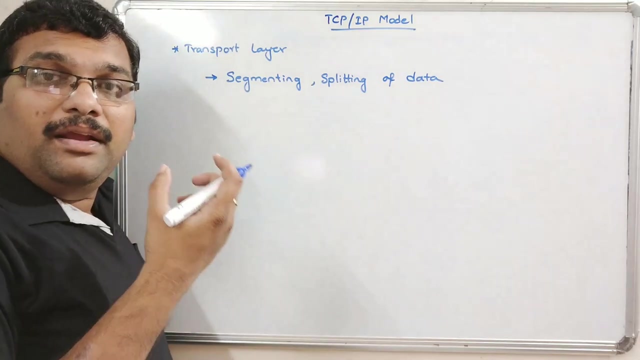 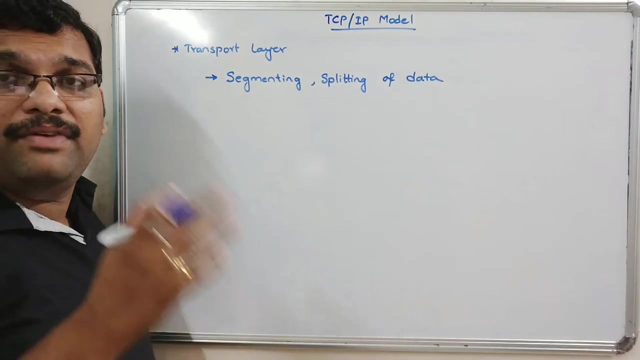 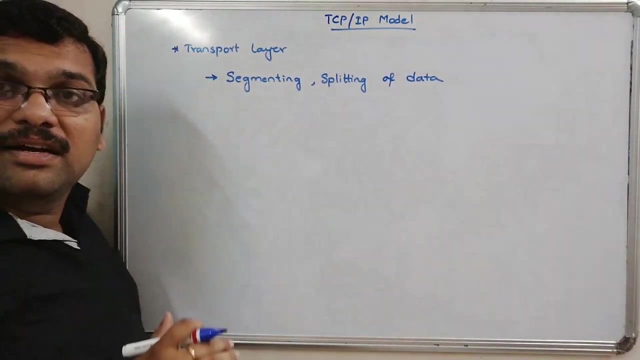 the, the, the, the. This is responsible for segmenting. splitting of the data, So the data will be divided into different segments. right So everything. splitting of data. So, based upon the bandwidth, the data will be divided. right, So everything that complete splitting of data is done in this transport layer. 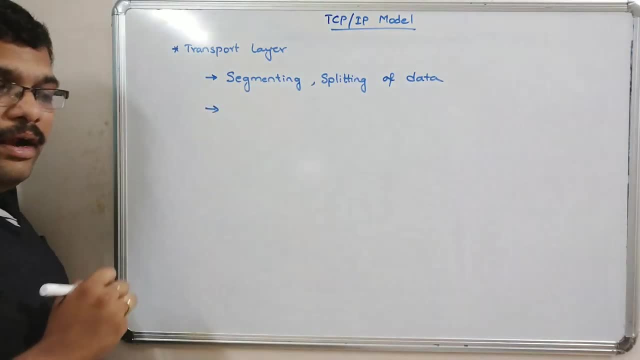 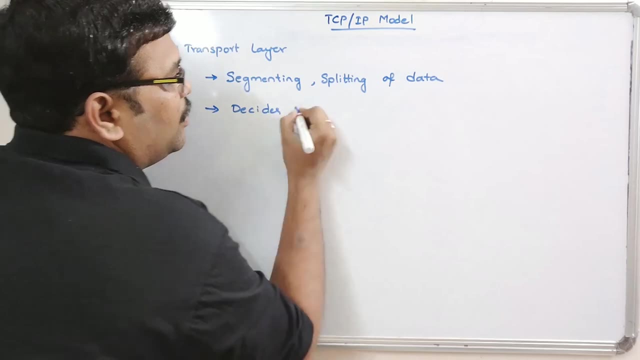 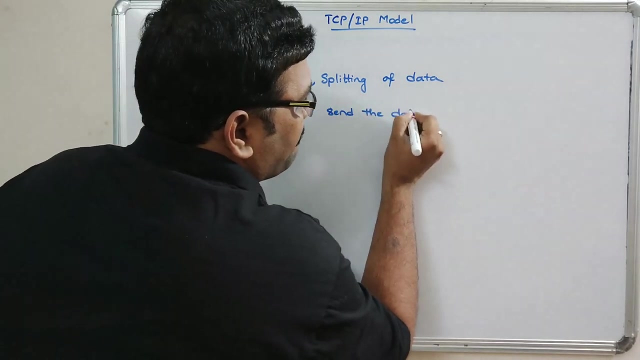 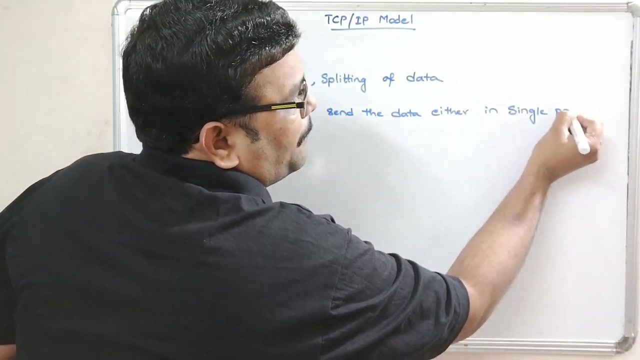 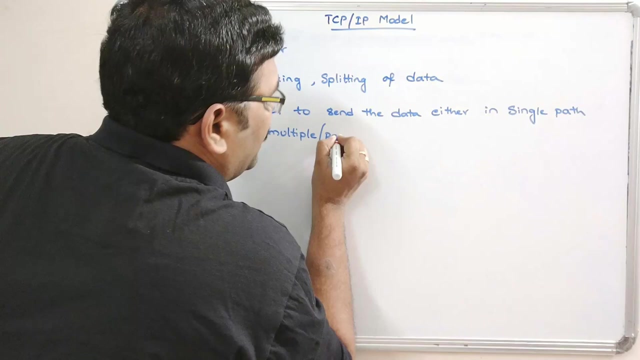 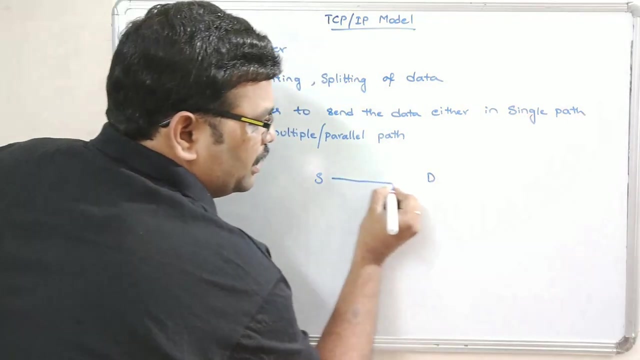 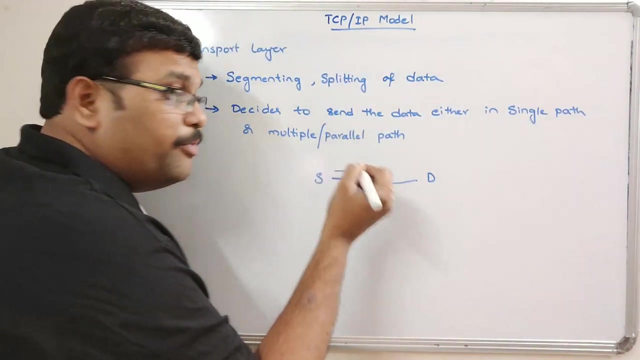 And it also decides to send the data Either in single path or multiple path or parallel path. That means source and destination, So it is then bidirectional. Source can send the data in this way And using the same communication channel. the destination should send the data. 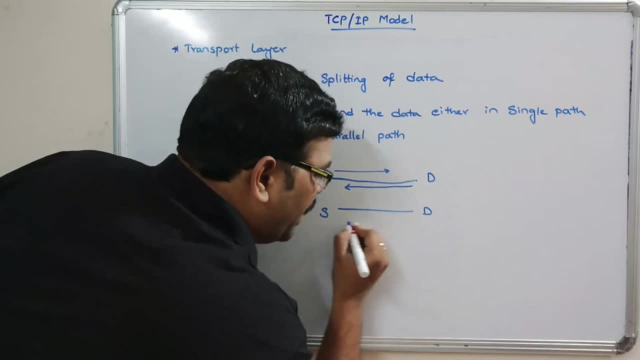 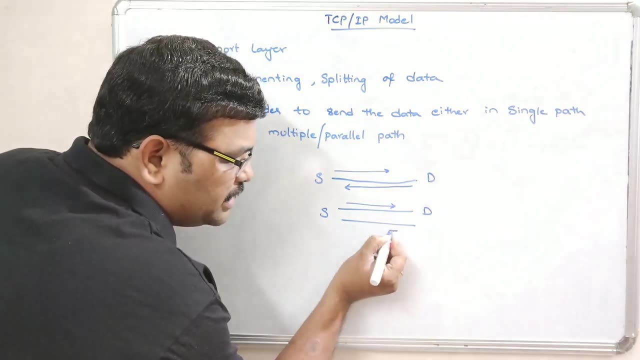 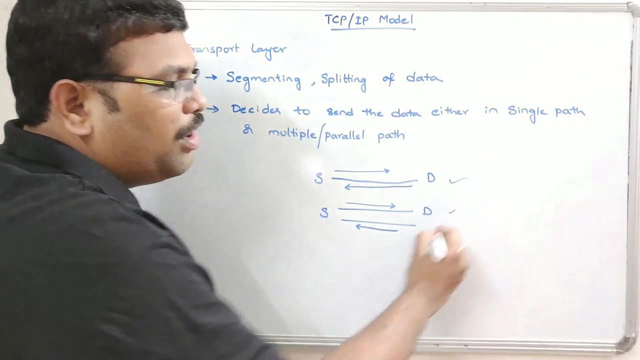 Or source and destination will be having two paths, So source can send the message in one direction from one communication channel And destination can send the data through the another path. So it decides to send the data either in a single path or a multiple path. 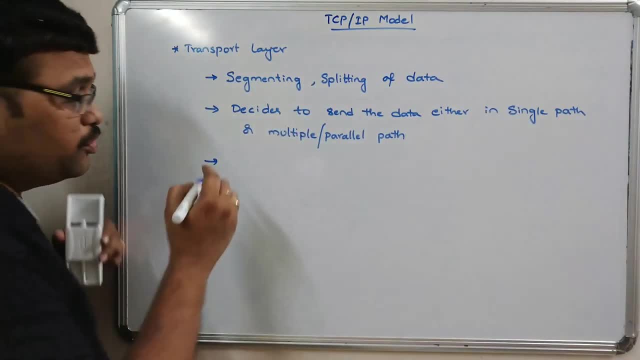 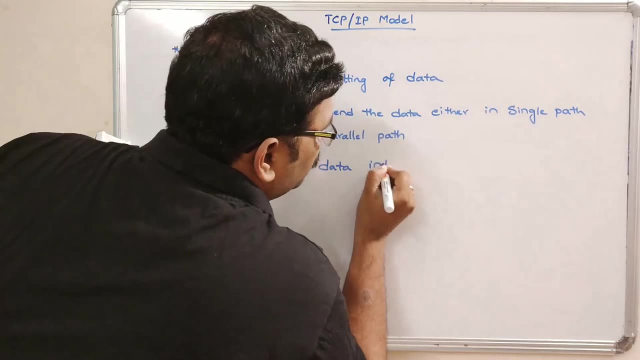 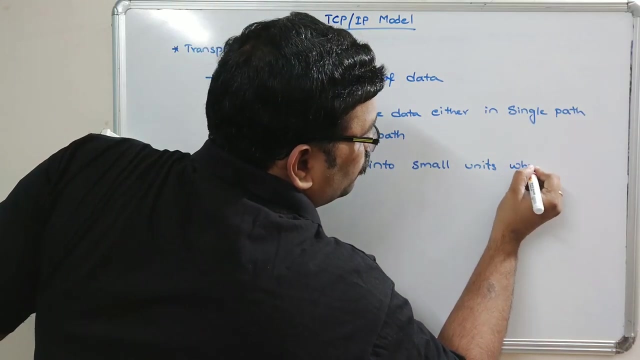 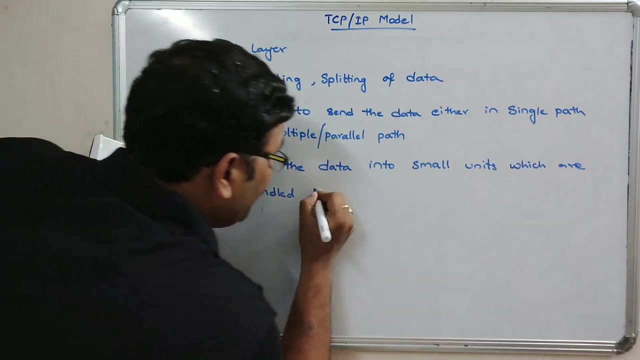 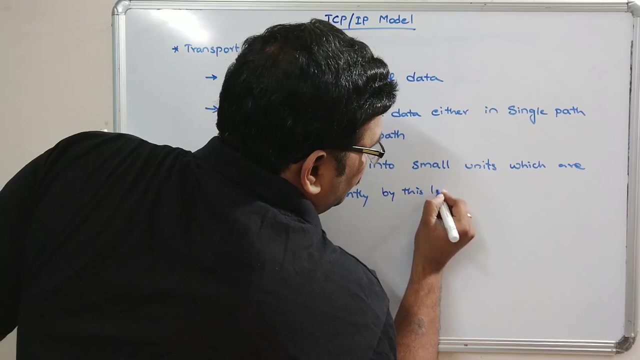 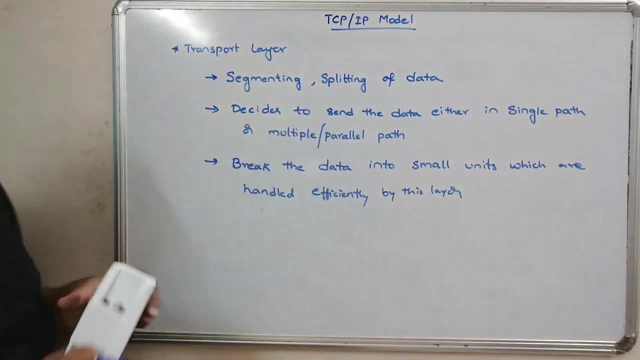 And this TCP-IP model used to bring Break the data into small units, which are handled efficiently by this layer. So, in order to handle efficiently, So in order to handle efficiently, The data will be divided into small units, right, And also, similarly, the header information will be added. 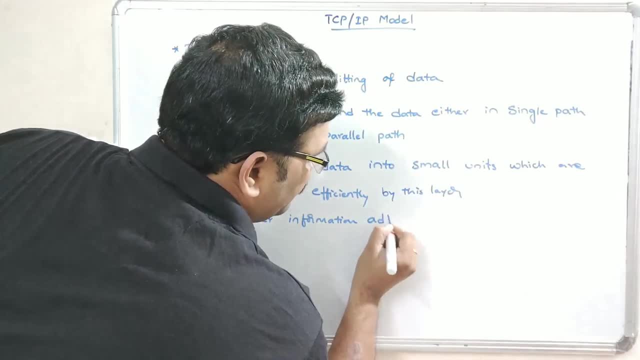 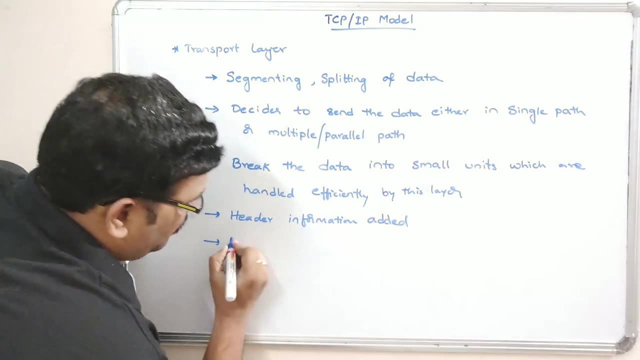 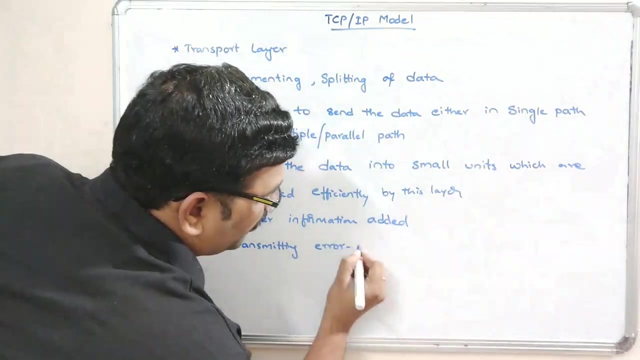 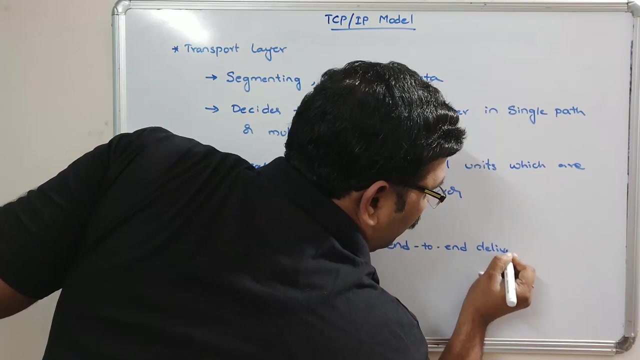 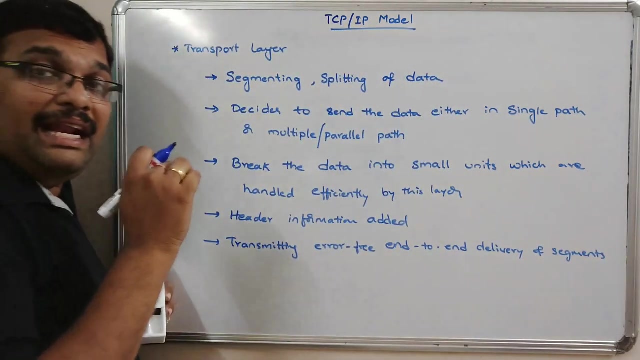 The header information will also be added in this layer And it is mainly responsible for Transmitting- Transmitting Error-free End-to-end Delivery of segments, So transmitting the error-free messages. this transport layer will be implemented. So hope you understood about this transport layer. 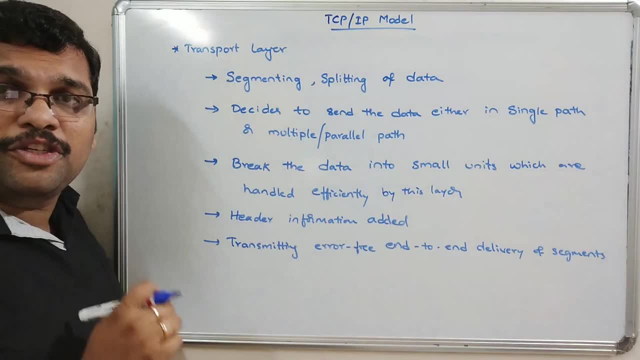 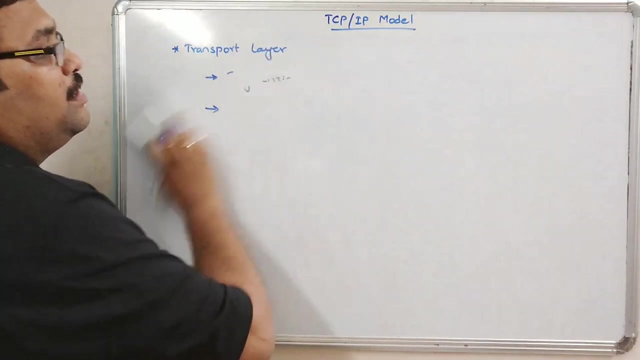 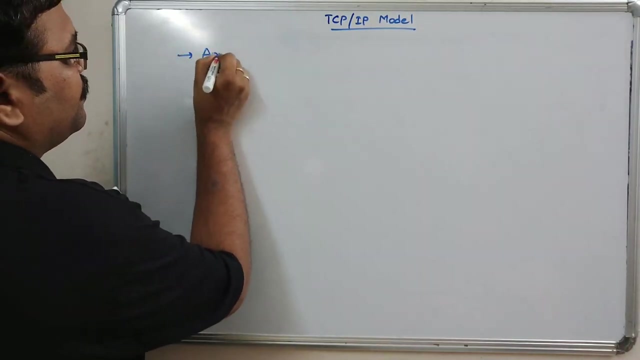 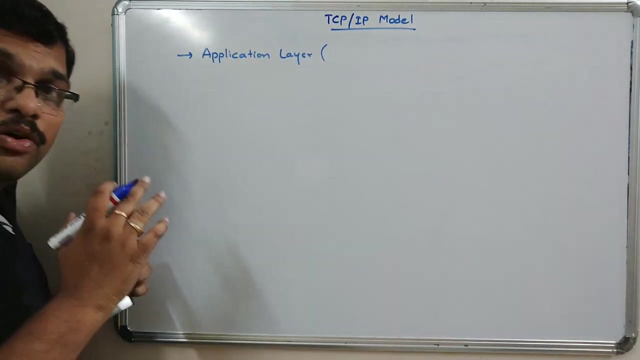 So one single thing. So, whatever the responsibilities and functionalities which we have seen in the transport layer of OSM model, Everything is applicable here, Right? So next, the topmost layer in TCP-IP is application layer. That means the combination of both the session and presentation. 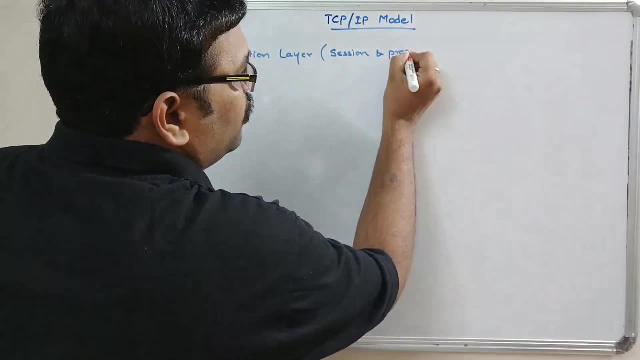 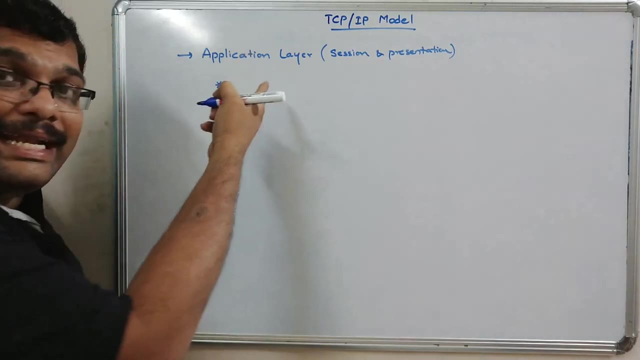 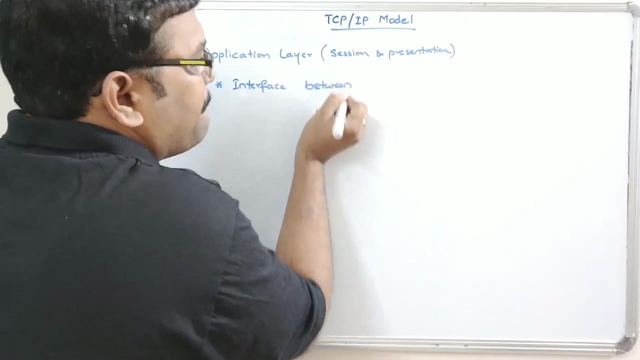 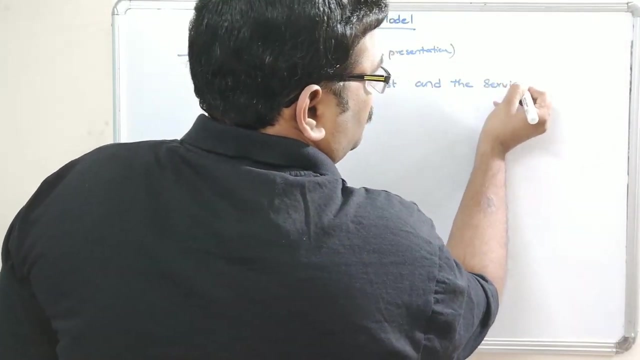 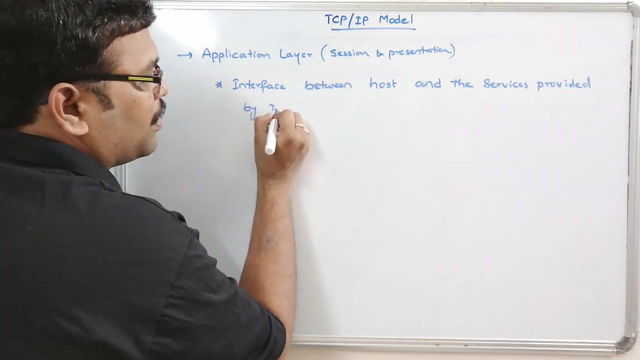 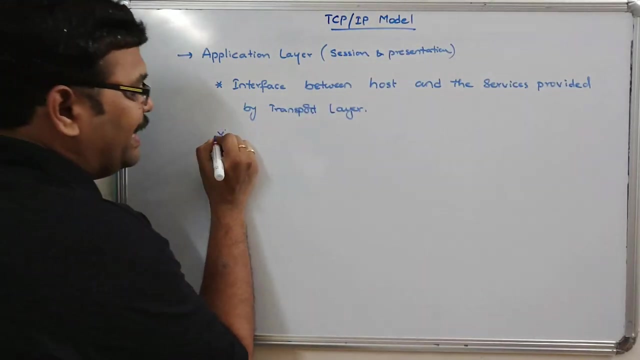 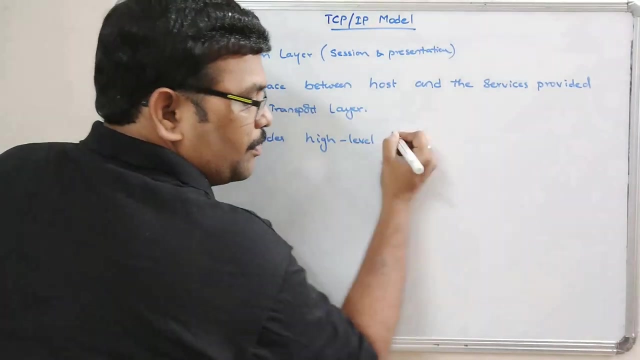 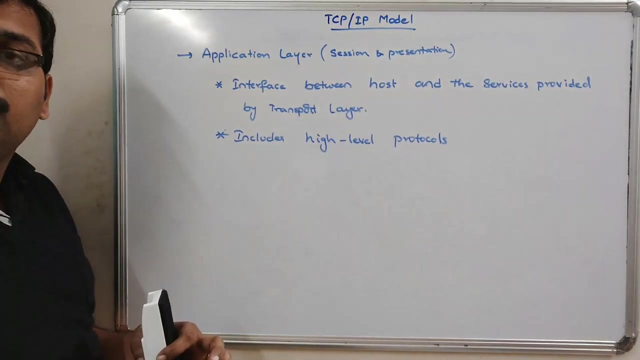 So session and presentation will also be included Right Here. it will act as an interface between the host and the services provided by transport layer Right. And also it includes high level protocols. It also includes the high level protocols. So what are the high level protocols which are involved in the application layer? 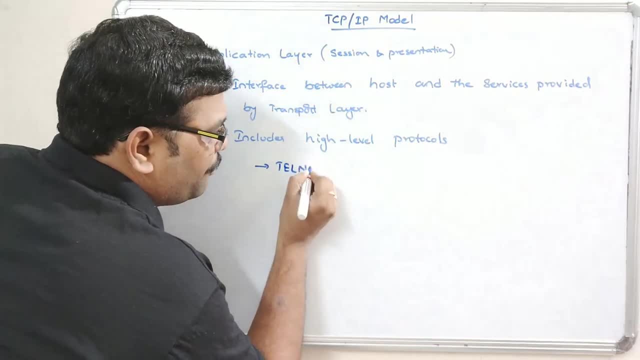 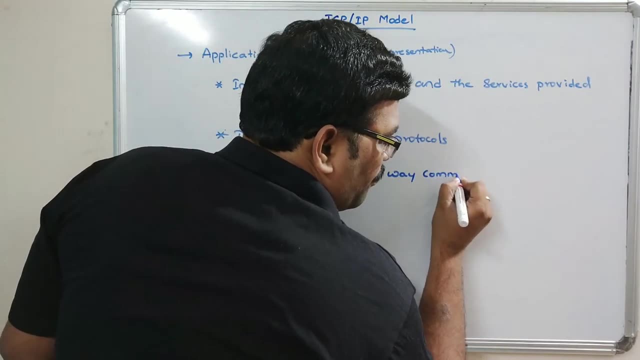 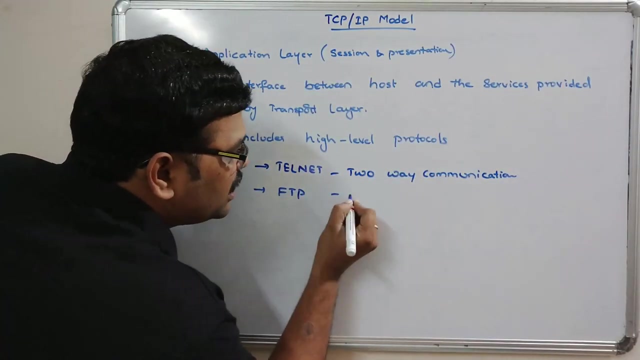 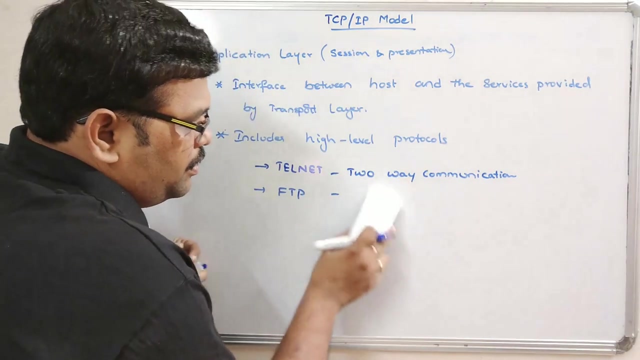 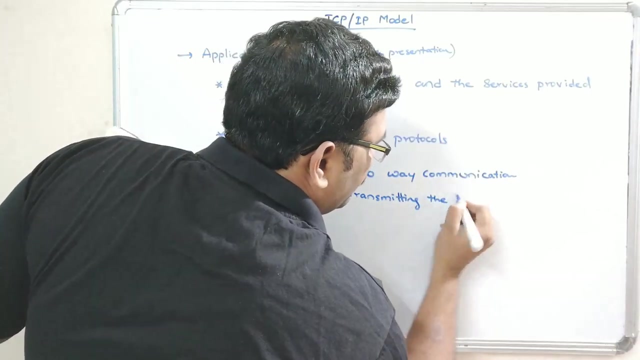 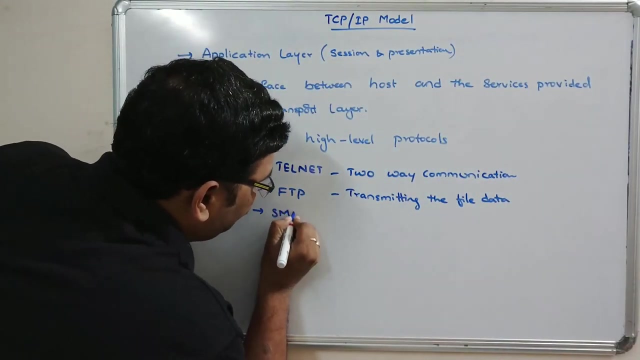 The first one is Telnet, Which is a two-way communication. Two-way communication And similarly FTP, Which is nothing but a file transfer protocol, Transmitting the data or file data from source to destination. Similarly, SMTP, Mail transfer protocol. 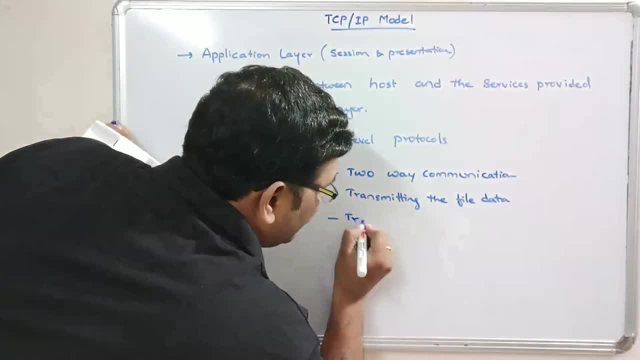 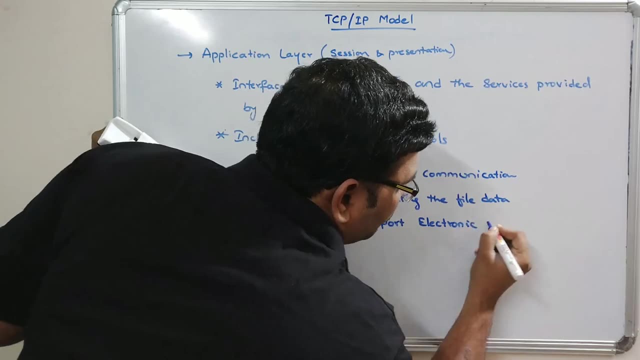 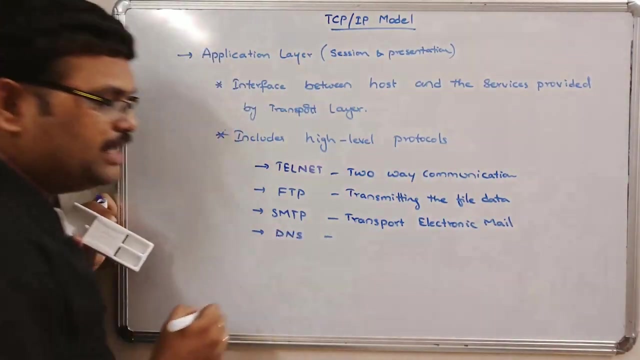 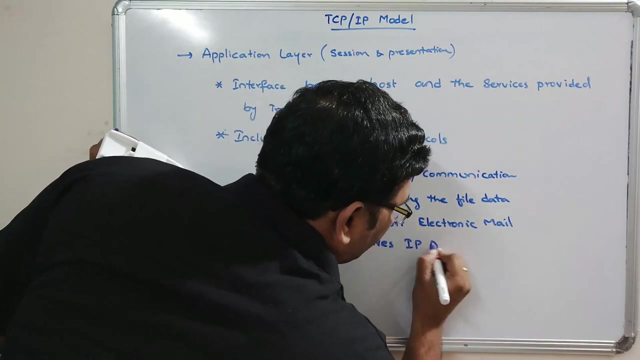 Right, Yes, Yes, Yes. Yes, That is a file transfer protocol. It is used to transport electronic mail from source to destination. Similarly, DNS. DNS is domain name service which resolves IP address to textual information. Yes, Yes, Yes. 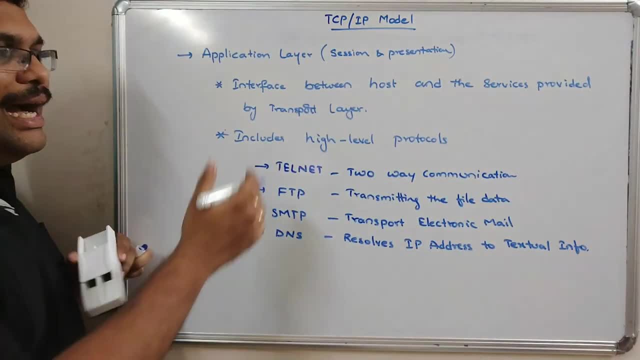 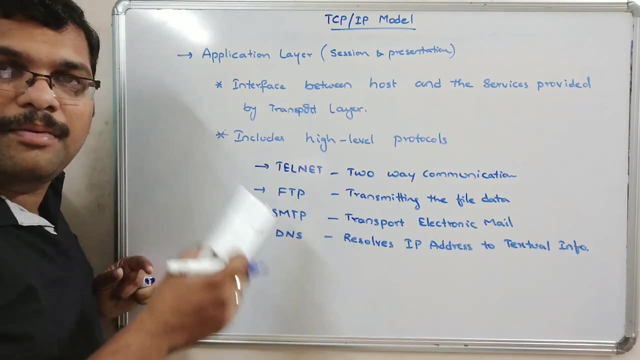 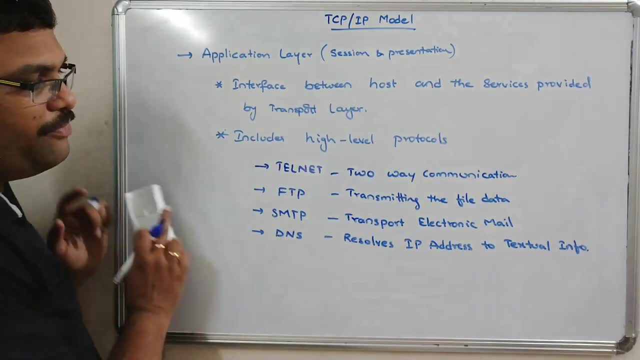 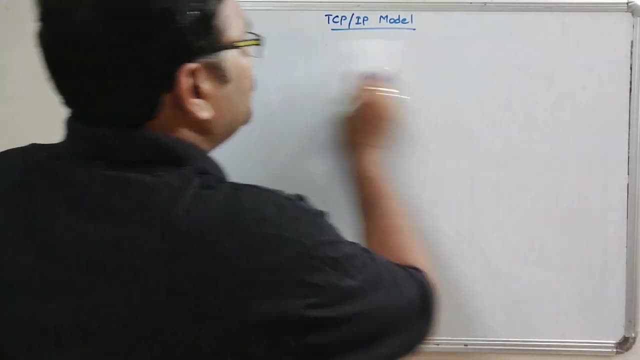 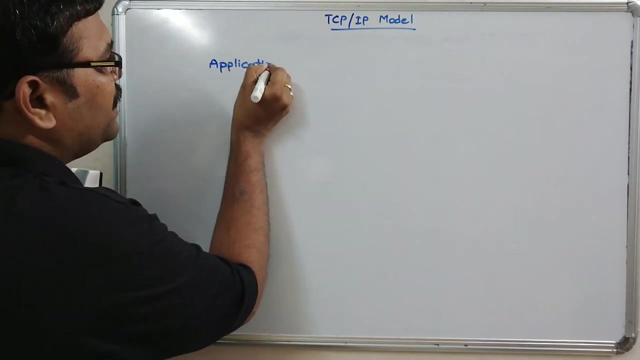 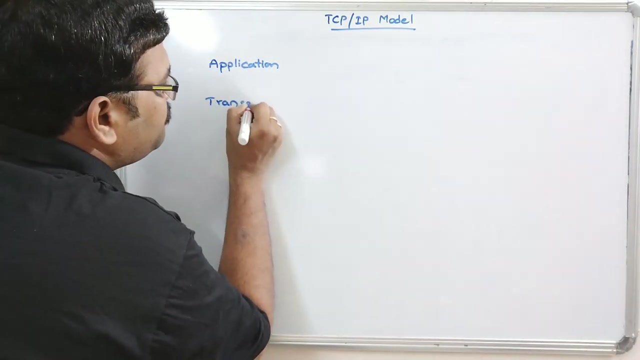 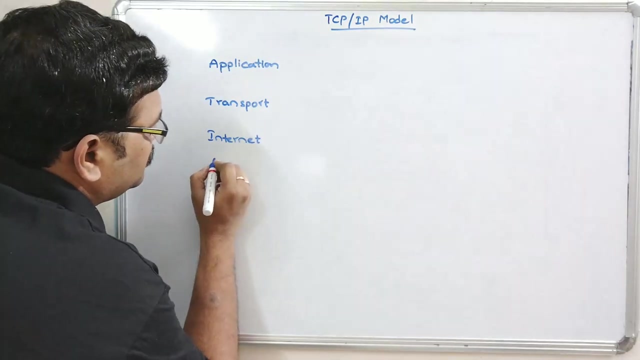 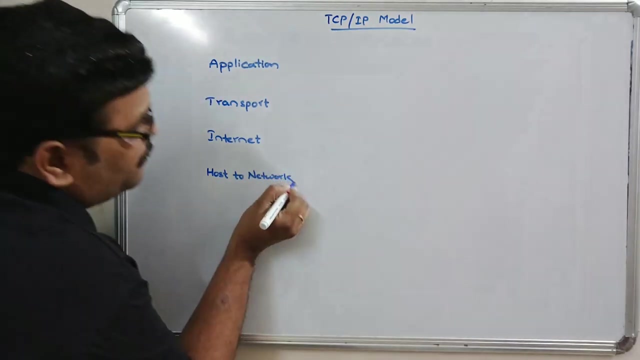 Now, finally, we will see the protocol stack of all these layers and we will wind up. See, let me give you the protocol stack for all the layers. So first, the top most layer is the application layer, then transport layer, internet layer, host to network layer. So the application, the protocols of applications are Telnet, FTP, SMTP, DNS, etc. In the transport layer we will use the two protocols: TCP, UDP, internet. the main protocol which we are using is IP protocol, host to host network. 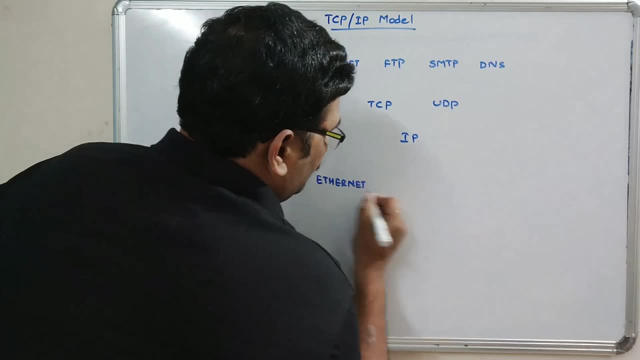 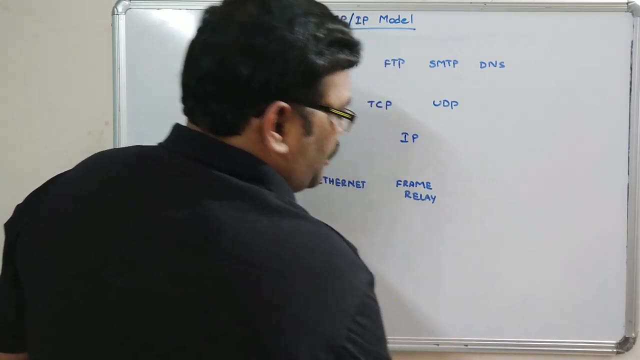 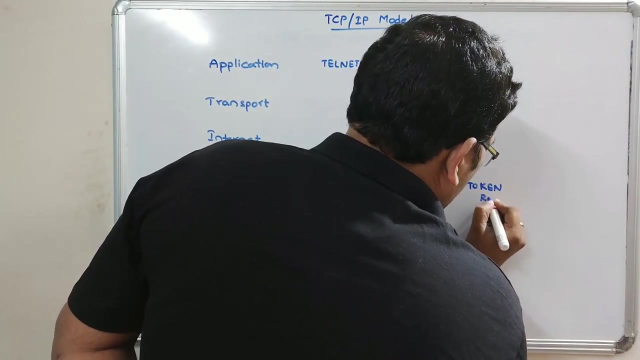 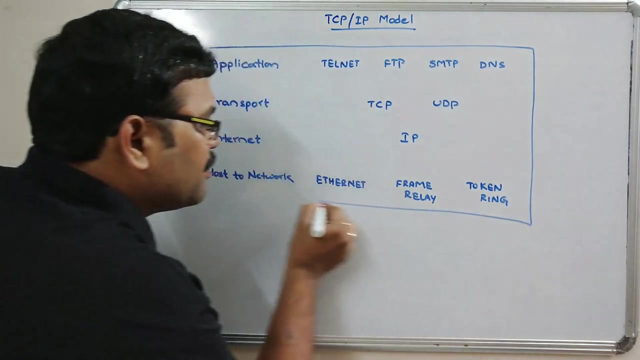 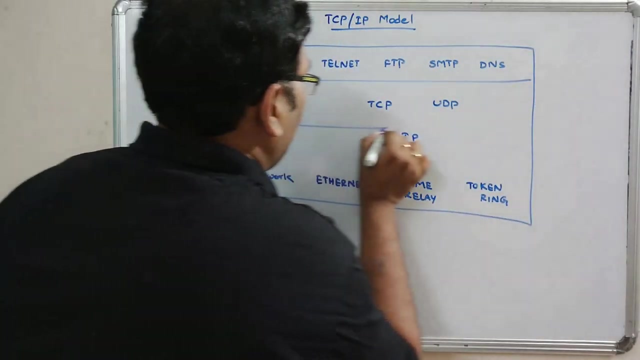 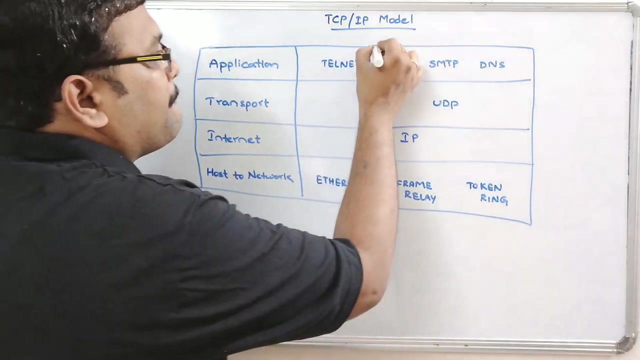 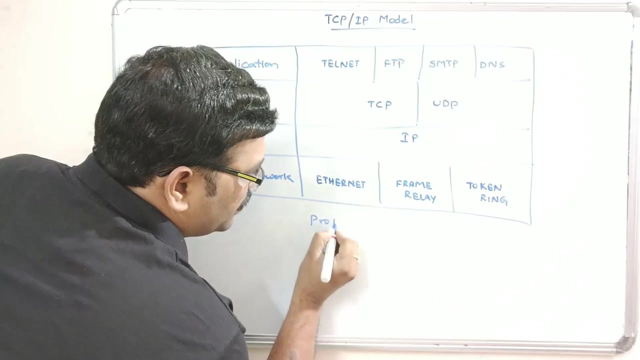 The data is Ethernet TCP Link, So it is the stack of all the layers which is included in this plataforma. You can seeue. you will see the protocol stack Andined Right. this is the protocol step, the protocols involved in each and every layer of this. 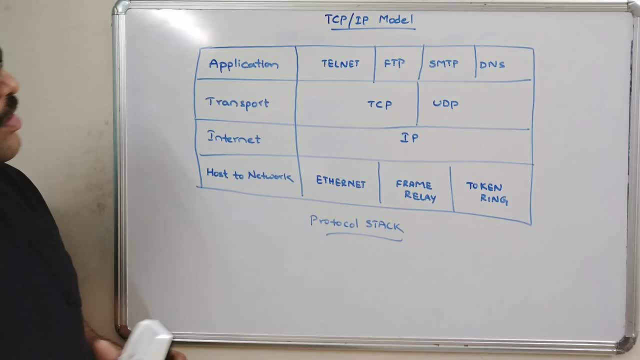 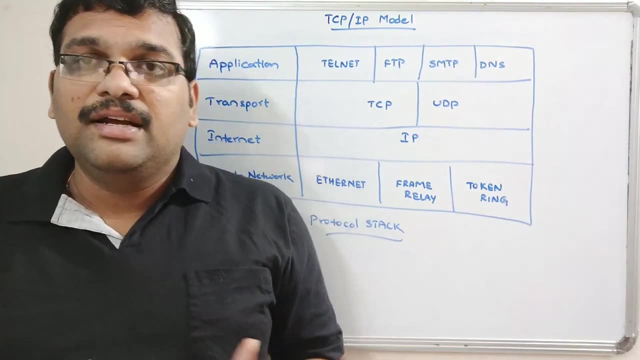 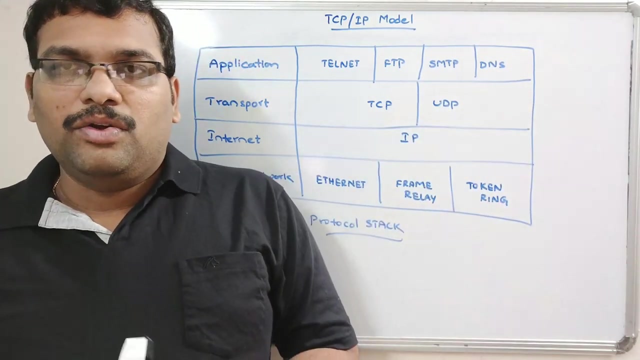 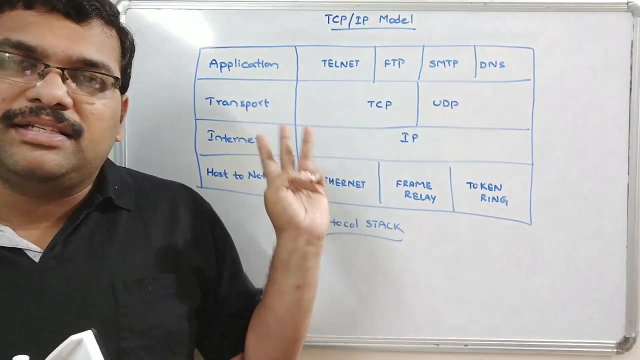 TCP IP model. okay, so hope you understood this TCP IP model. the only one difference over the OSI reference is that is a reference model and that is this. TCP IP is an implementation of that OSI model. so one more difference of this TCP and OSI are it will be having. OSI is having seven layers, whereas this. 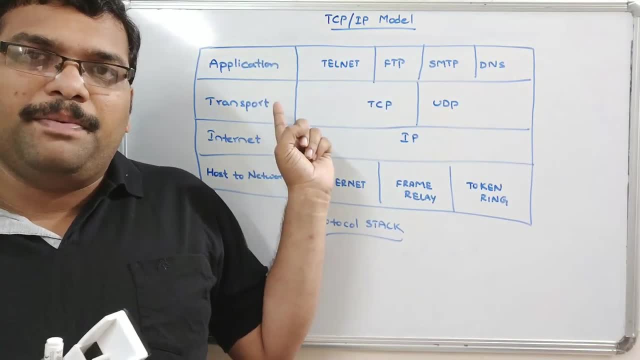 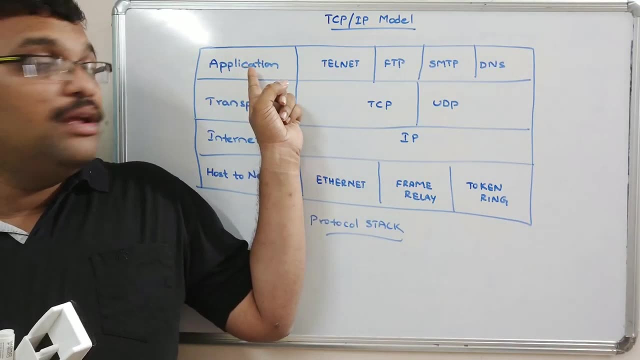 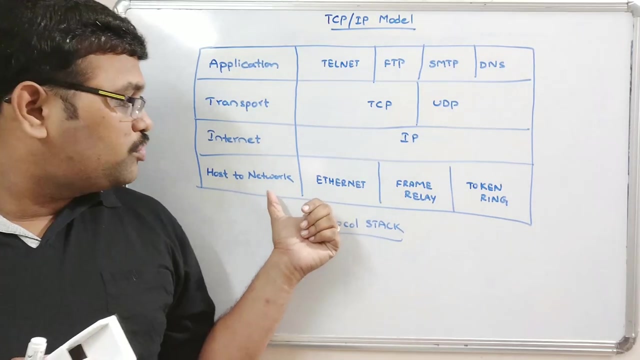 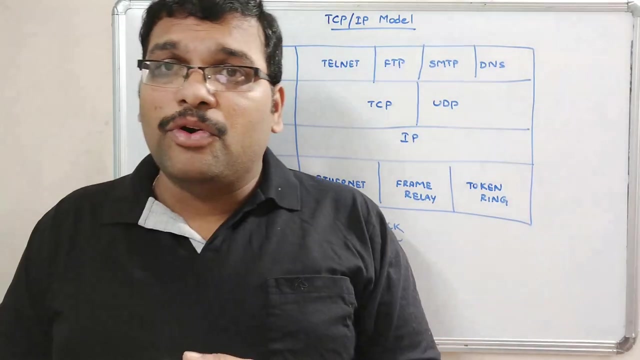 TCP. while implementing the OSI, this TCP IP reference model is having only four layers, so the session layer and presentation layer are combinedly combined into application layer. similarly, the physical layer and data link layer are combined into the host to network layerAnd one more difference is this TCP IP modal supports only connection-less. 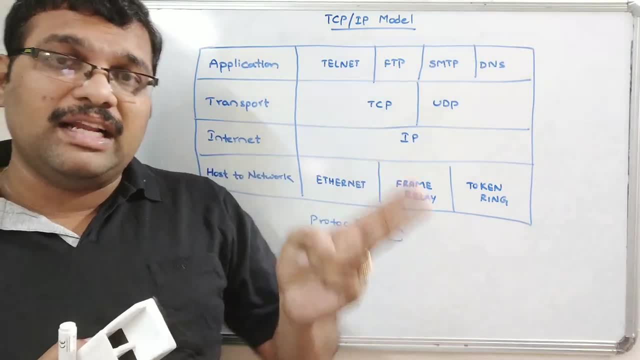 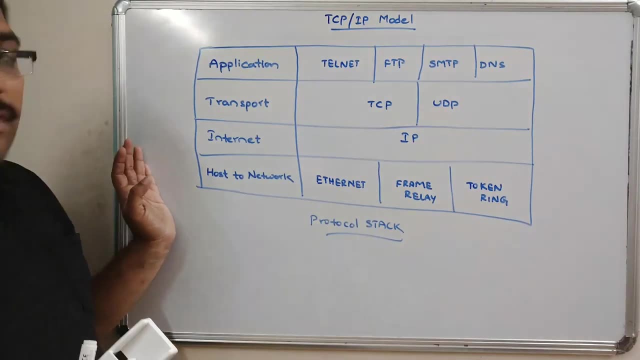 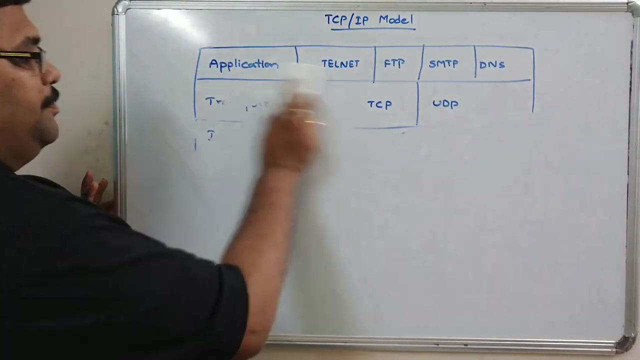 service well, as OSI supports both the connection less and connection-oriented sans right. So let us write the difference of this: TCP IP is the connection-less version and the OSI version. the OSI service is not. we can calculate the and OSI reference model and then we will stop this session. 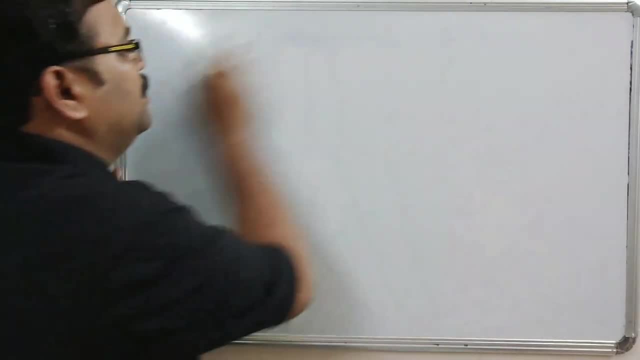 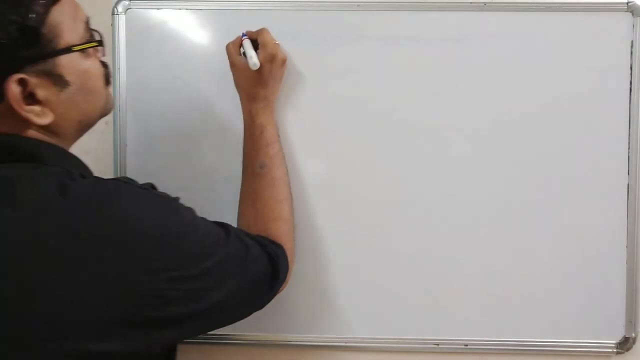 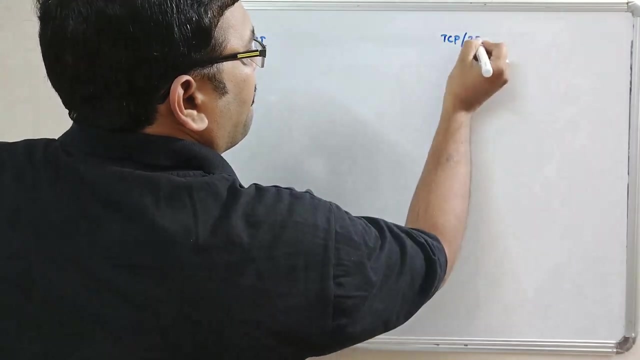 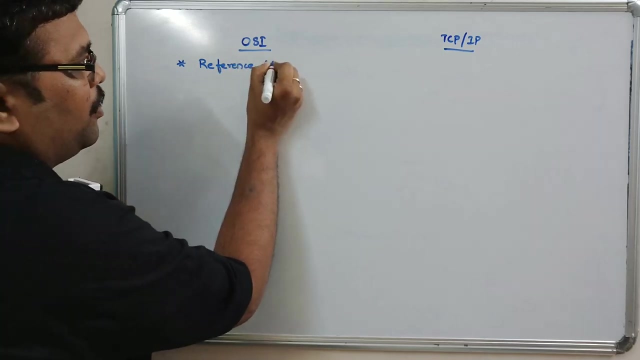 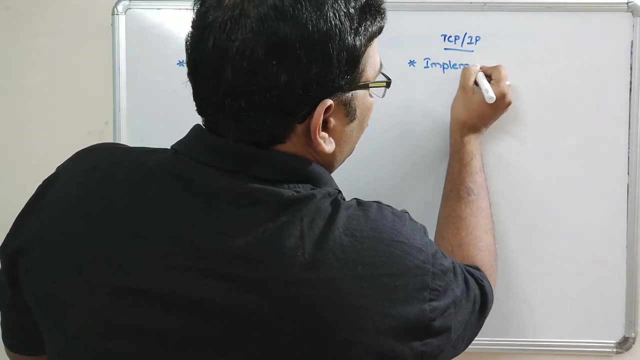 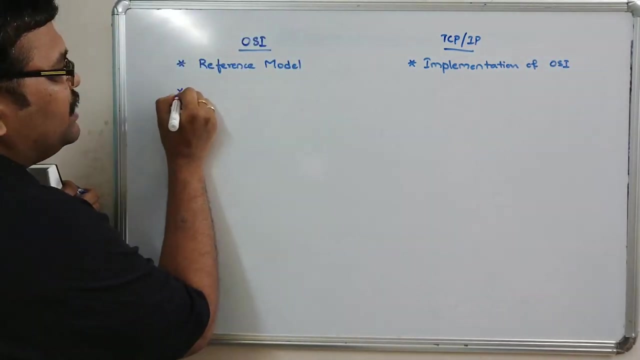 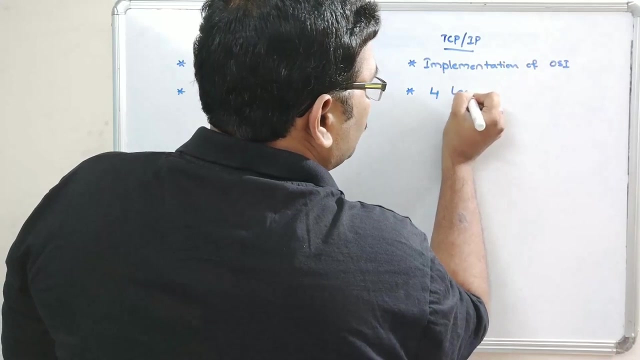 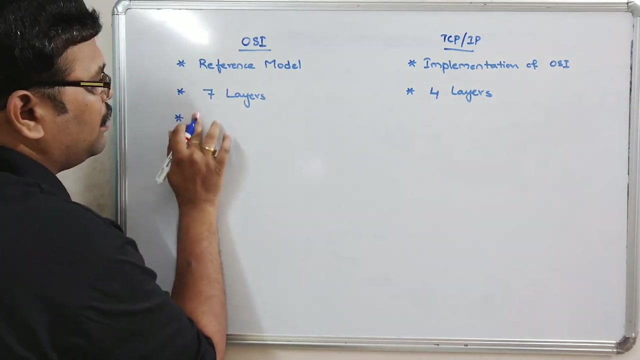 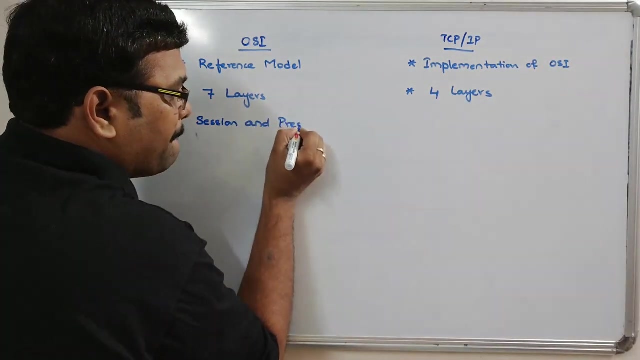 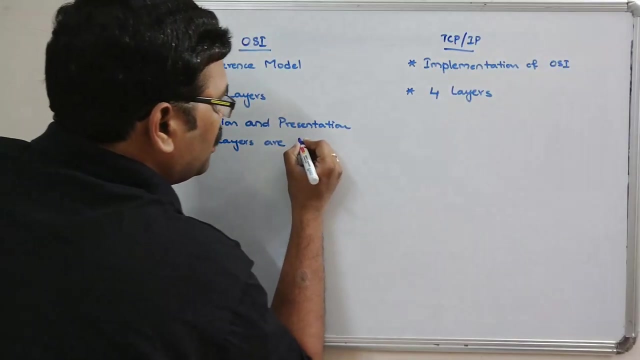 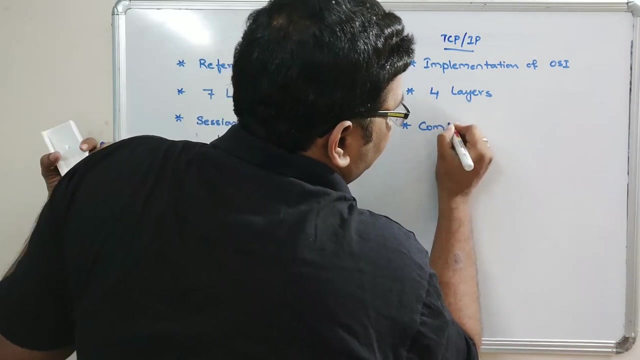 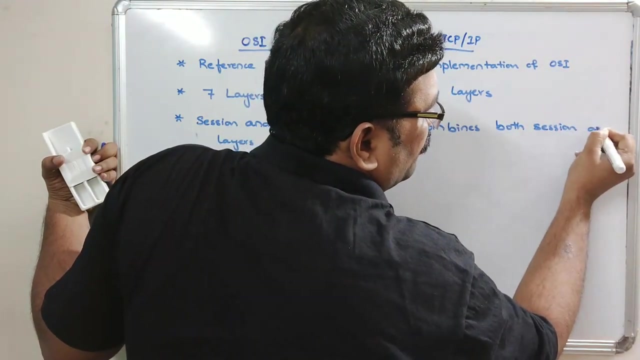 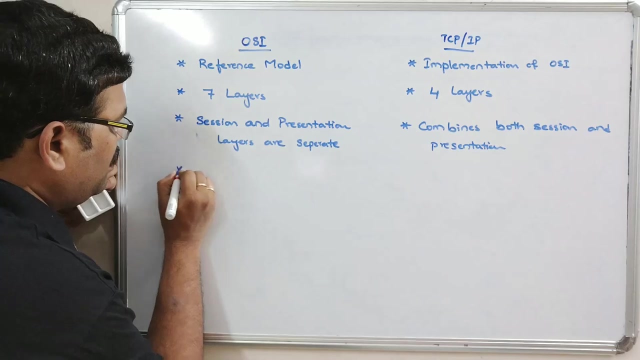 right. so first one is it is a reference model and here we have seen it is an implementation model of OSI. so this will be having seven layers and this is having only four layers, and here the session presentation layers are separately implemented. here it combines both session and presentation layers here.